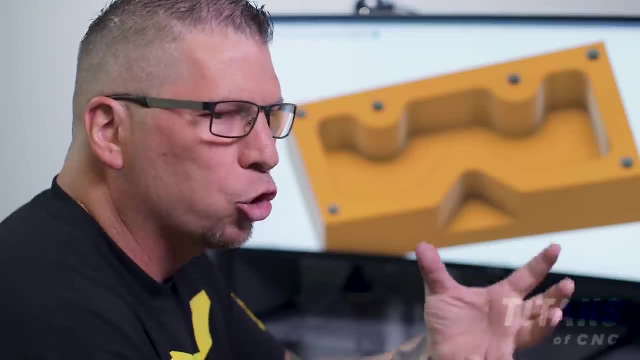 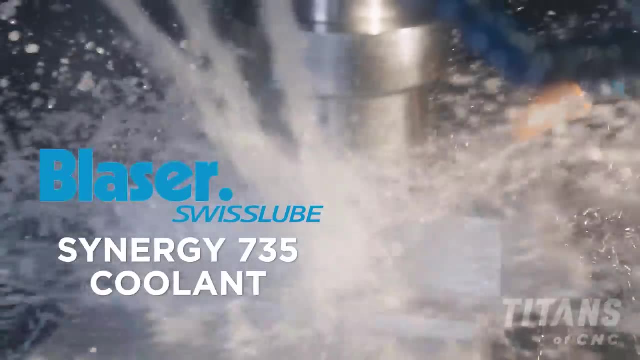 cut a material with a high nickel content, the cooling, the lubricity, all of it comes into play, and the cooling can literally make you or break you. So you need a different tool, You need a different approach. But then when you step up and cut a material with a high nickel content, the cooling, the lubricity, all of it comes into play. 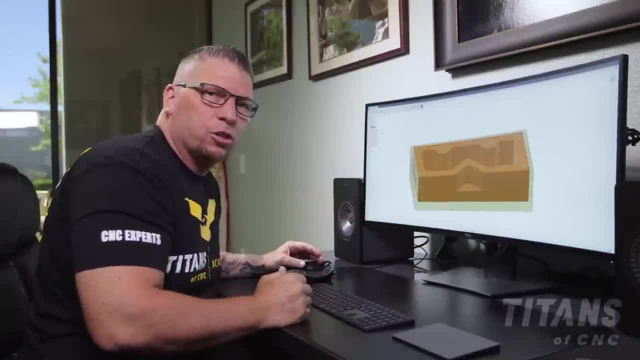 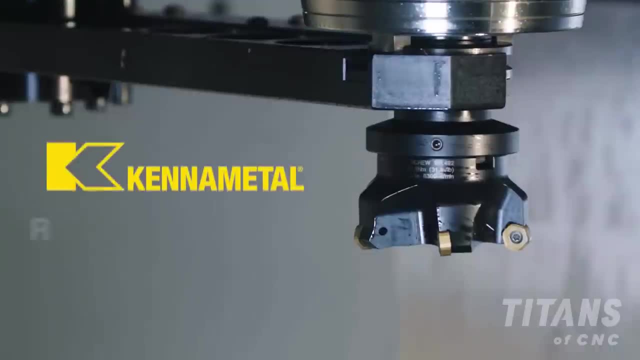 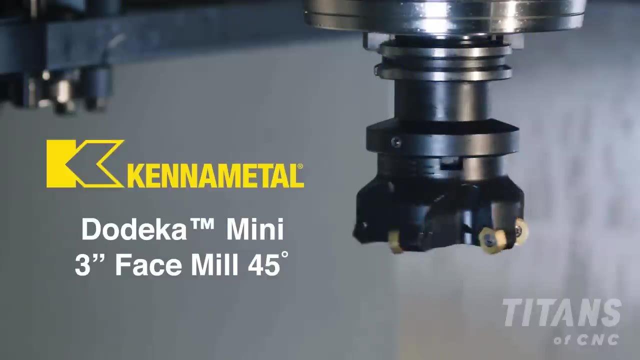 and the cooling can literally make you or break you All right. So the first thing that we're going to do is actually cut the top surface of our part, And to do that we're going to use a three-inch Dodeca Mini Shell Mill. So the insert that we're using is not the insert that I used. 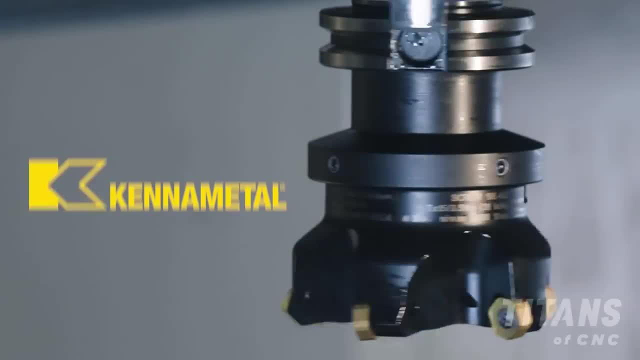 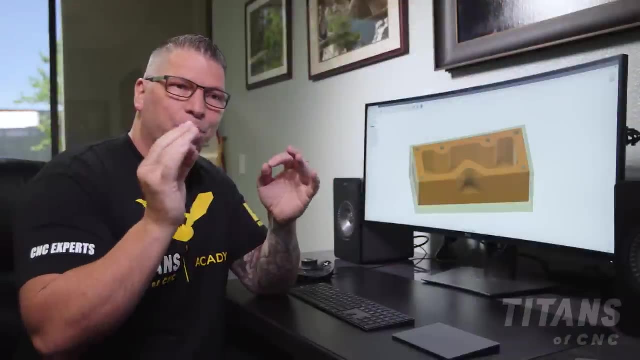 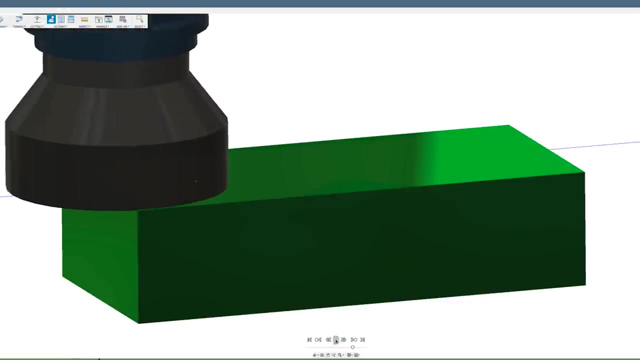 10 years ago. This is a new insert. This is the KCSM40.. It's a special blend of carbide So you can machine a perfect part consistently. So we're using this Shell Mill to create the first datum, the first perfect surface, And then when 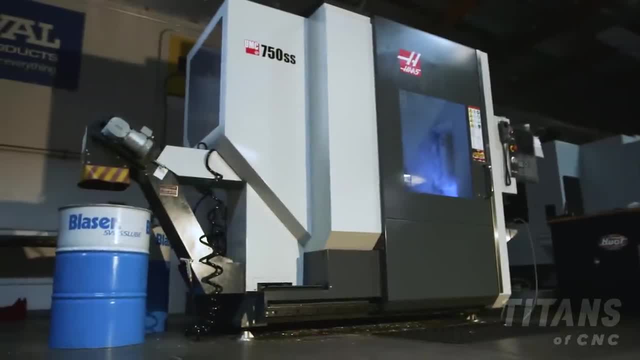 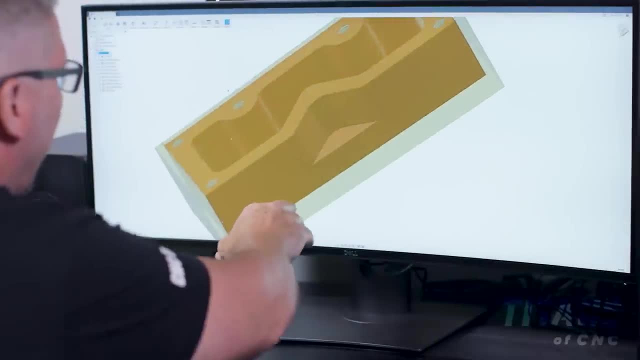 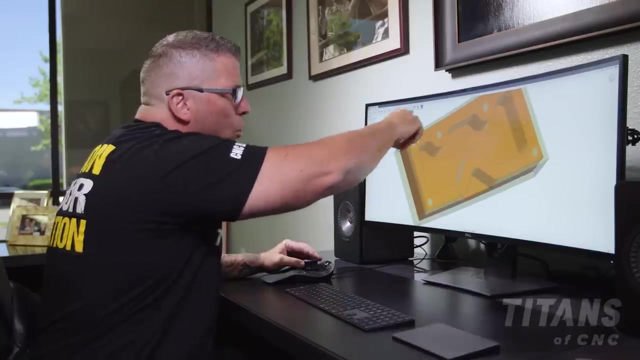 we drop down and create pockets and holes, all the dimensions will come off that surface. So you see the part right here. I got my excess Inconel, the material I'm holding on to on the outside, And then I got material all the way around and I got material on the top. Okay, So if we're 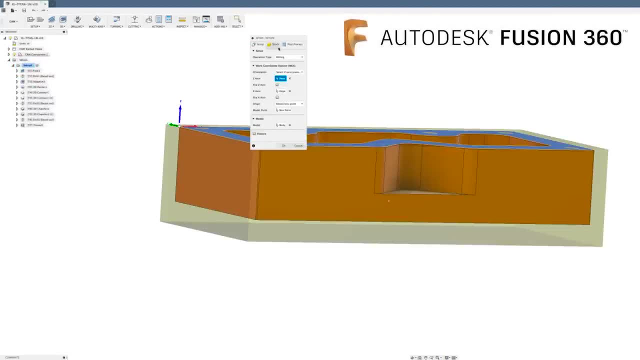 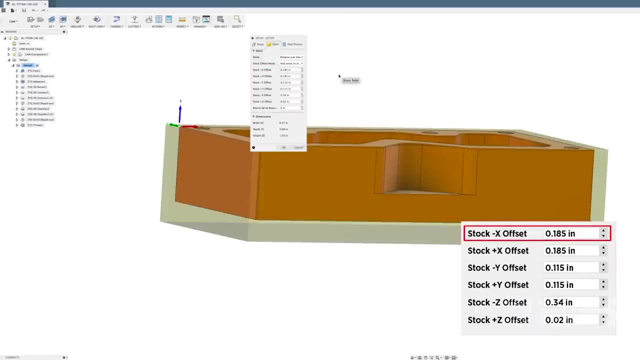 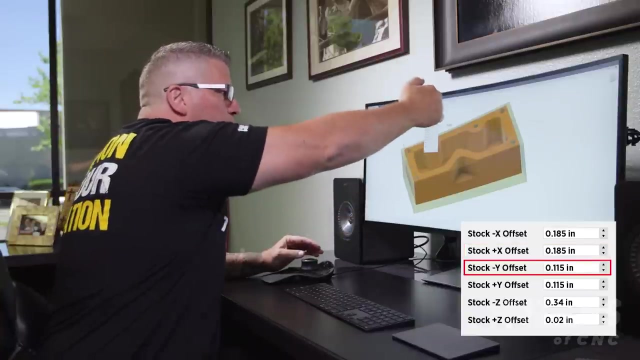 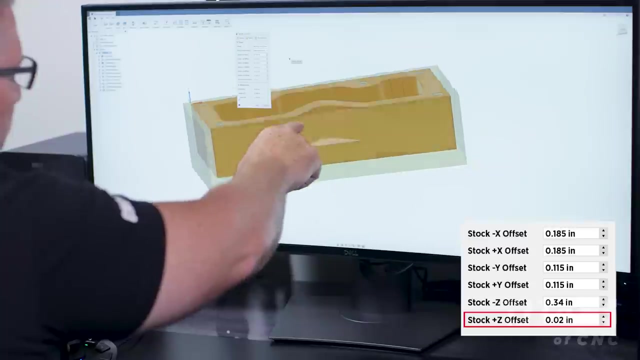 going to actually go into my setup and go into edit. come to stock. you can see exactly how much material I've left. So we have 185 thousandths on X negative, X positive, 115 thousandths in Y, So 115 in the back, 115 up front. I have 20 thousandths right here on the top surface. 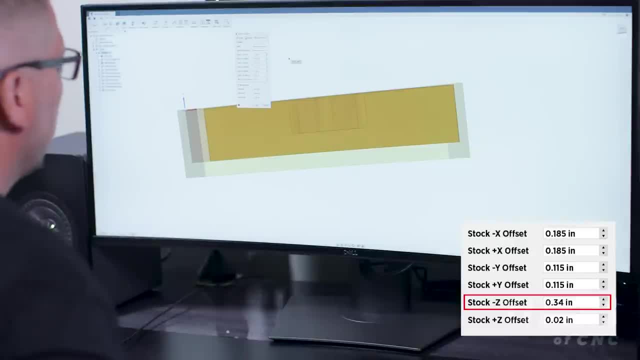 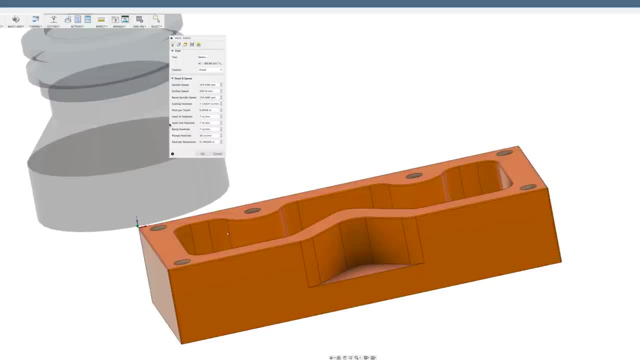 And I have 340 thousandths on the bottom surface. All right, So let me explain the speeds and feeds for the Dodeca Mini. We have a surface foot of 200, which has given us an RPM of 254.. And we have five inserts on. 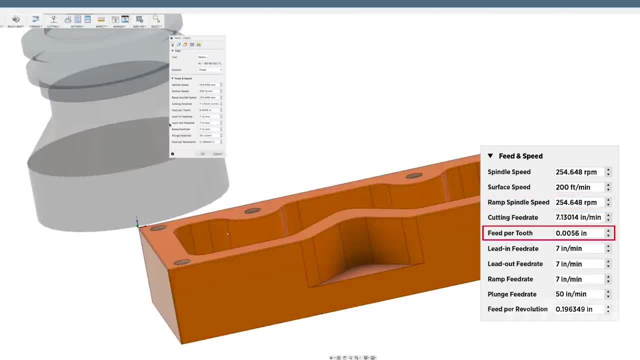 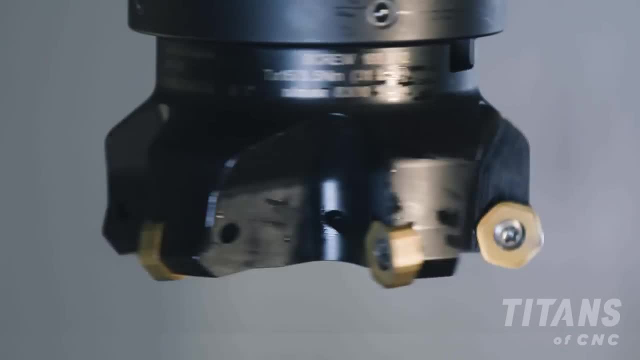 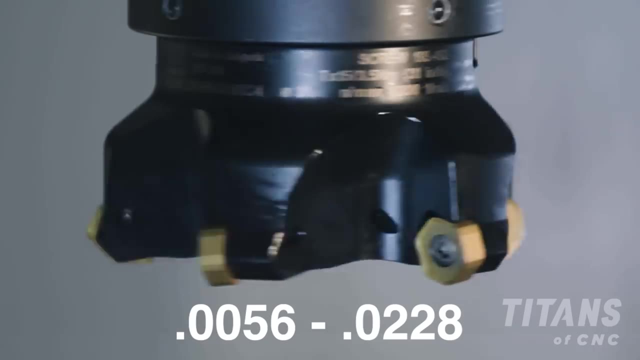 this Shell Mill. So when you look at our actual feed per tooth, 0056 is way on the bottom, because the range on this specific tool and insert is 0.0056.. 2.0228.. So, as you can see, we got sky on the other side. but since this is a tutorial, 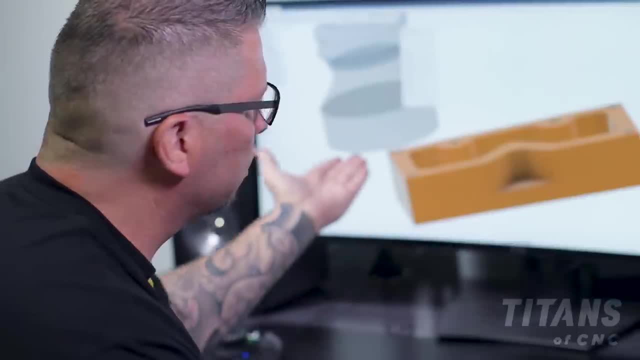 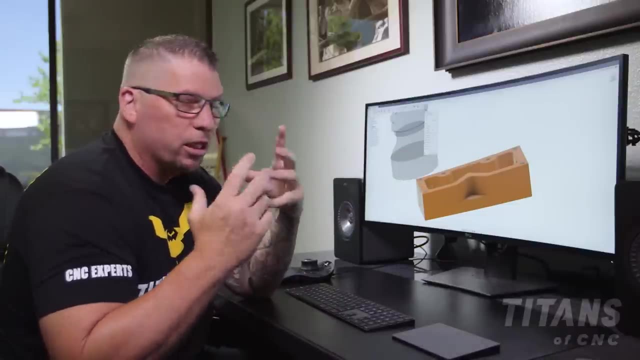 I wanted to slow things down, All right. So on this pass we're just taking a little bit of material on the top, but it is Inconel and we want to have a beautiful surface finish. So another thing that I've done is we've taken one insert out, brought in a wiper. 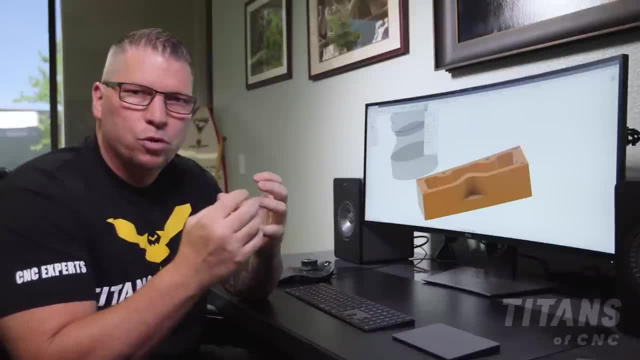 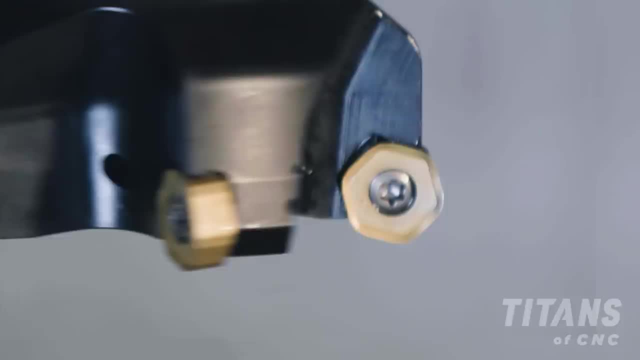 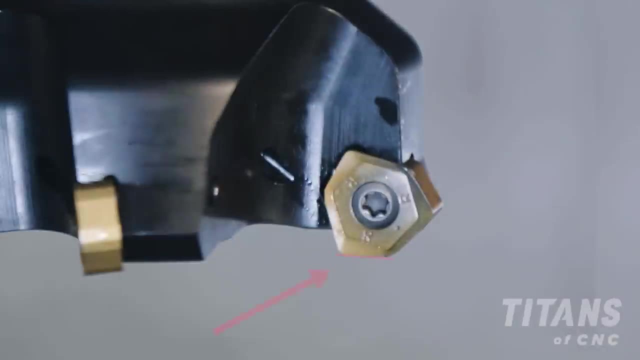 So what is a wiper? So it's an insert that we use to clean out a beautiful surface finish. So all the other inserts actually come down and have a radius at the bottom. that actually is cutting the material. The wiper actually has a flat on the 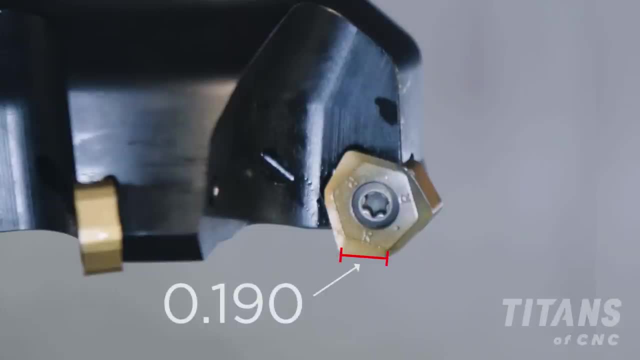 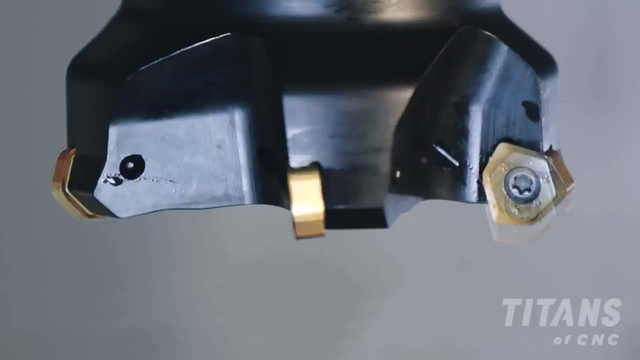 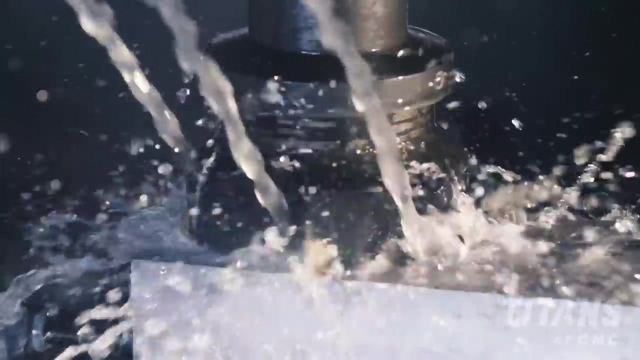 bottom. The flat is about 190 thousandths wide and the wiper actually sits lower than all the other inserts. So if the inserts were at zero, the wiper would be set down at 0.0028.. All right, So that's the difference between the two, And what happens is the first. 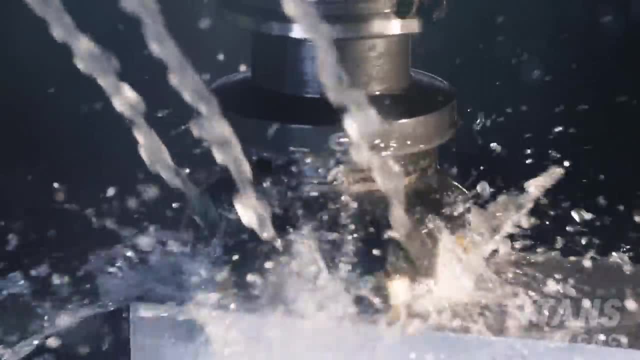 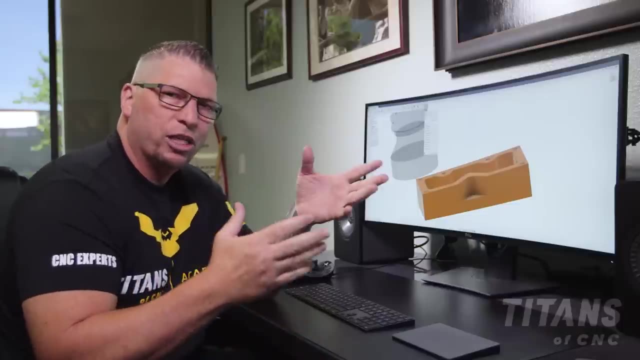 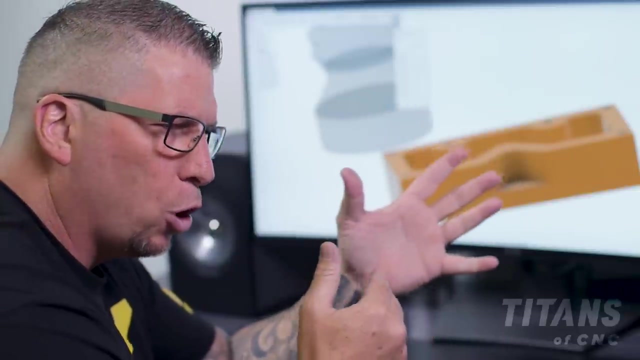 four inserts are going to come and cut the metal and then the wiper is going to come back and clean, All right. So we're starting out with 200 surface foot, but on the machine I might raise it a little bit to get a little bit more RPMs, And then I will adjust my chip load to slow or speed it up. 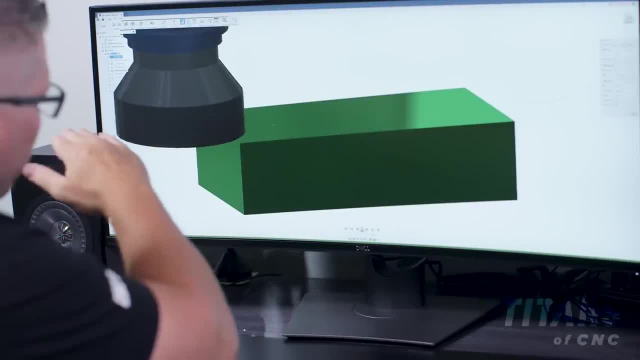 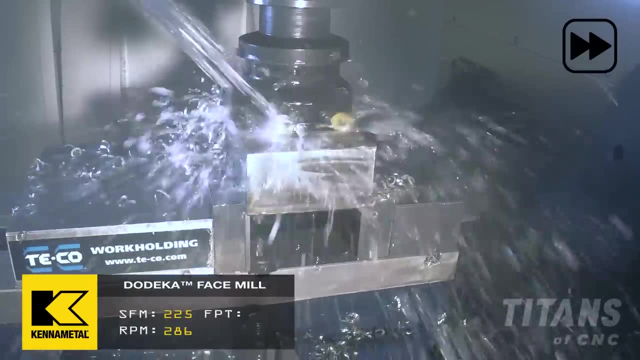 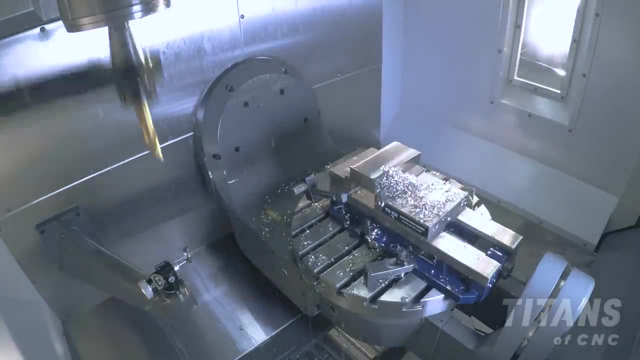 to get that perfect finish, The shell mill comes across and just skims perfectly across that surface. All right, So the first tool is complete. Now let's go to the next tool. The next thing I'm going to do is actually come down and actually rough out this pocket. 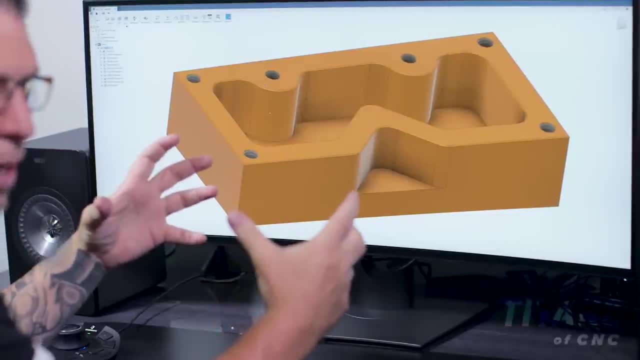 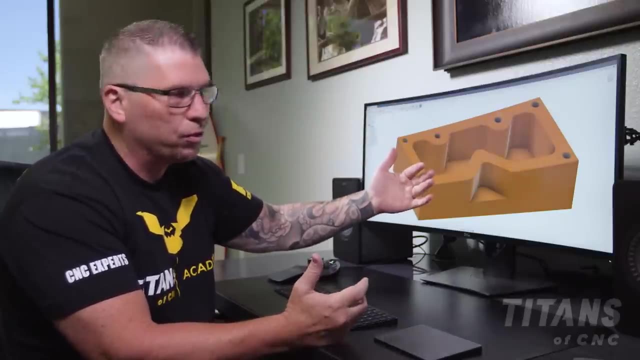 rough out all the material and start bringing the part to shape. I know that bringing an end mill into this ink canal straight down is a problem. right, We can helical and put a lot of wear on the bottom of that tool and possibly. 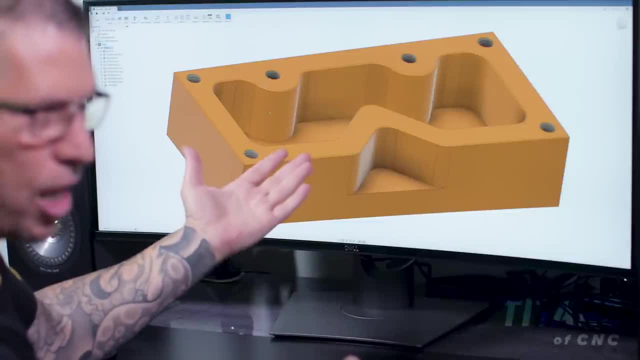 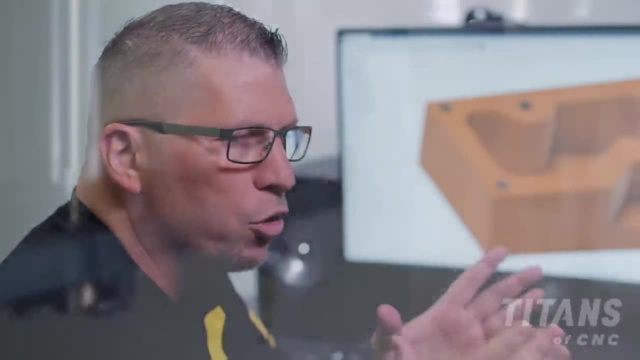 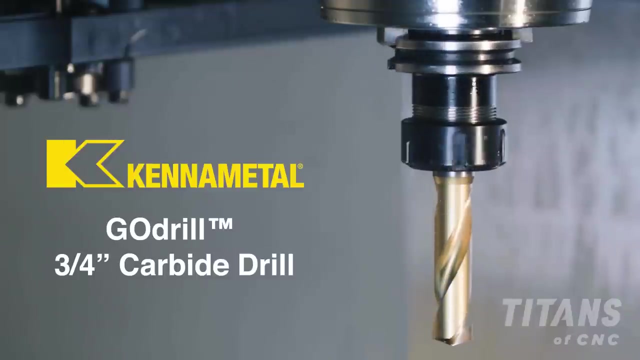 get it done, But that also is going to take a long time. So to solve that problem, I'm going to take one of my multi-purpose drills that I use all the time, the GoDrill. This is a solid carbide coolant through drill that can pretty much drill anything, So from steels to stainless to titanium. 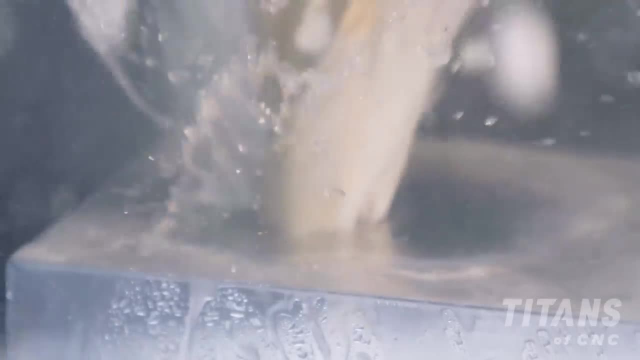 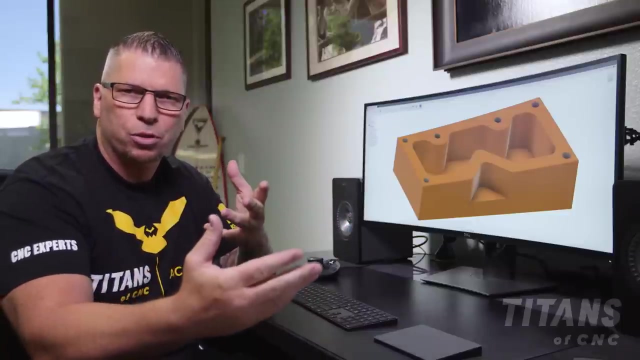 to ink canal monel. This drill. it can get the job done. If I was going into production and I was running thousands of parts, I'd probably go to an insert drill right, Like the Ken tip or the Ken tip FS or. 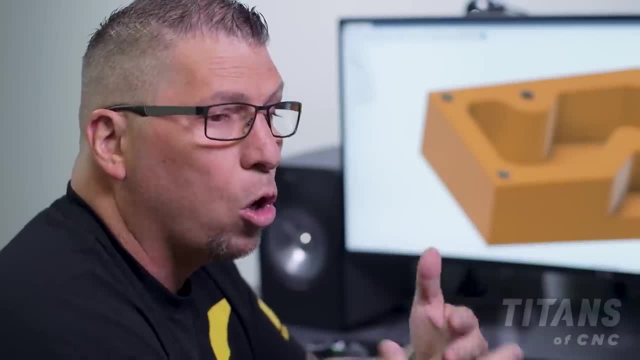 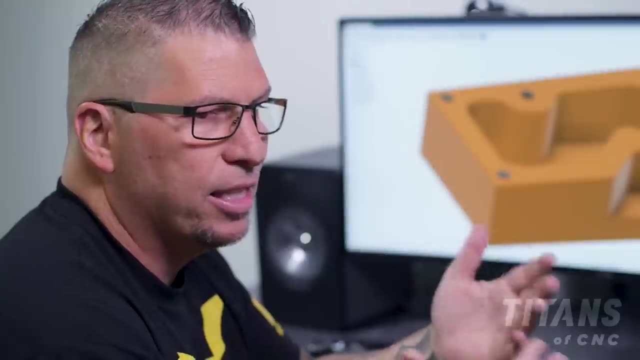 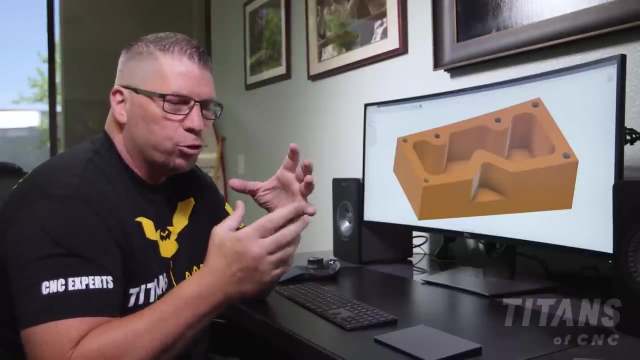 something similar. So once the tool got dull, all I would have to do at that point is change out the insert, which is a lot less carbide to pay for and makes it affordable. In this case, the GoDrill is the perfect choice. So the reason that I'm actually using a drill is to 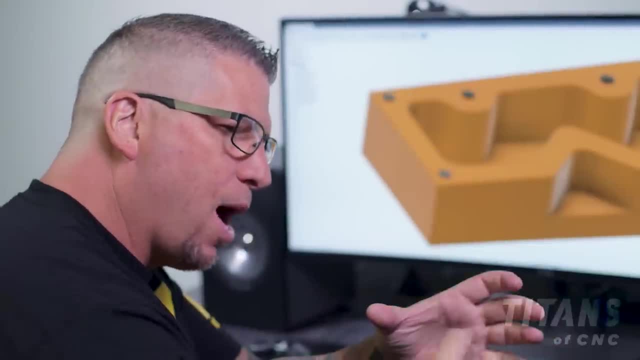 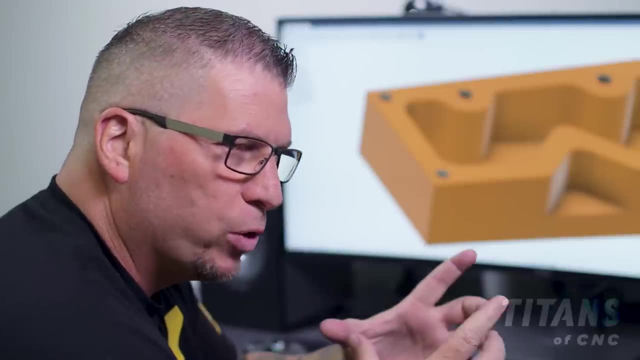 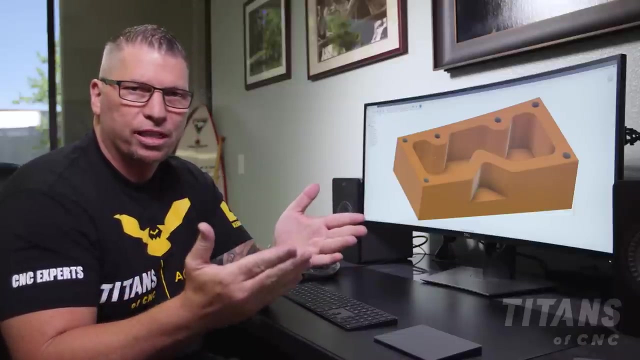 pre-drill, where the end mill is going to drop down into the pocket. So my end mill is going to be a half an inch. I just need a bigger drill diameter than the end mill. So for the GoDrill I'm going to use three quarters of an inch. That gives me an eighth of an inch all the way around. 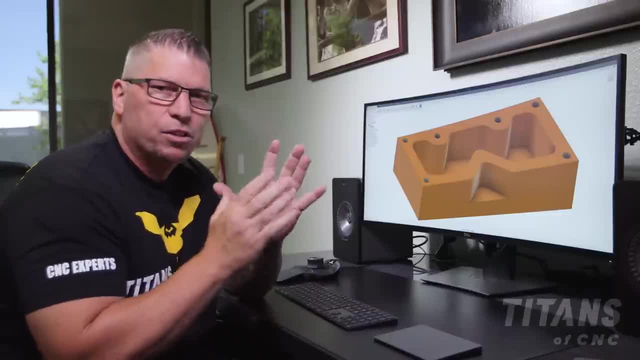 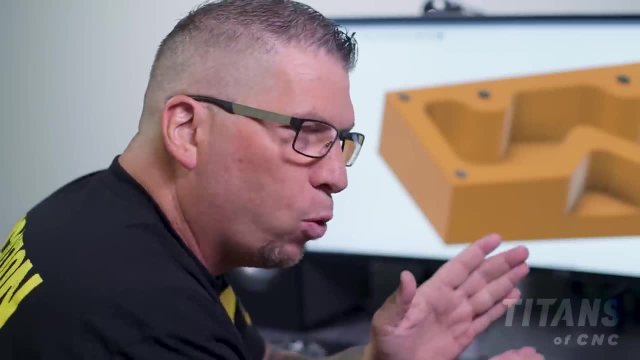 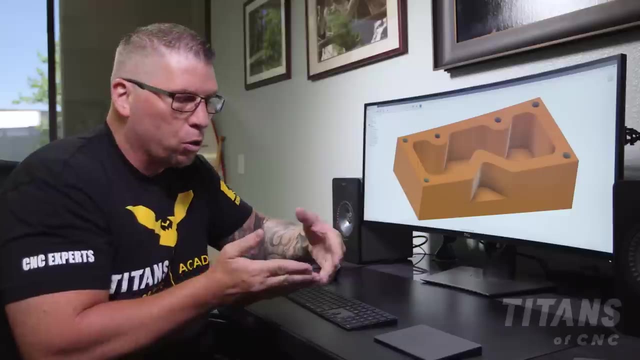 for clearance. This is extremely important because when the drill drills it's going to leave a tape or bottom, because the drill point is not flat. It's at an included angle at 140 degrees. So when the end mill drops down it's actually going to hit the tapered material before it hits the bottom. 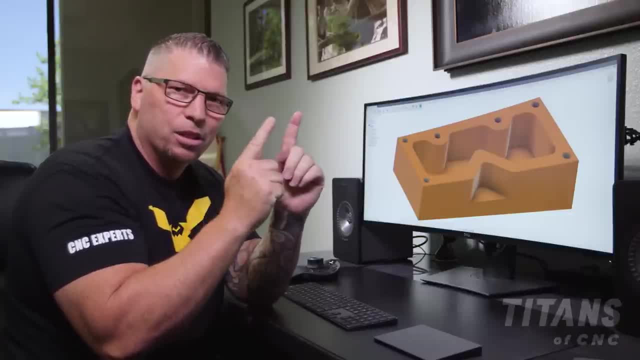 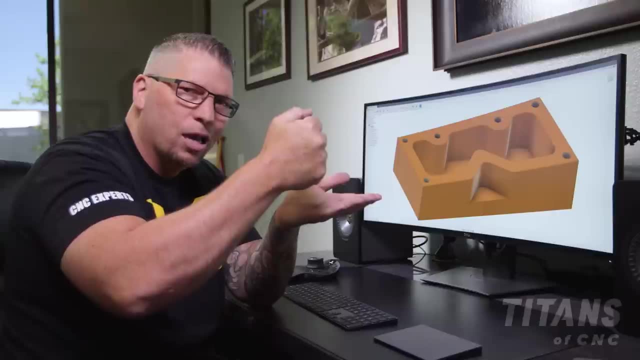 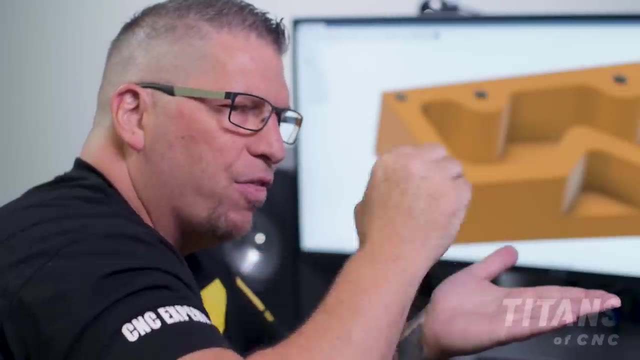 So, because I have a bigger drill than the end mill, when I'm about a hundred thousand shy of hitting the bottom, I'm simply going to step over at like 110 thousands And I'm just going to heal it cool Down to full depth at that point. Once I get to full depth, I'm going to start peripheral milling. 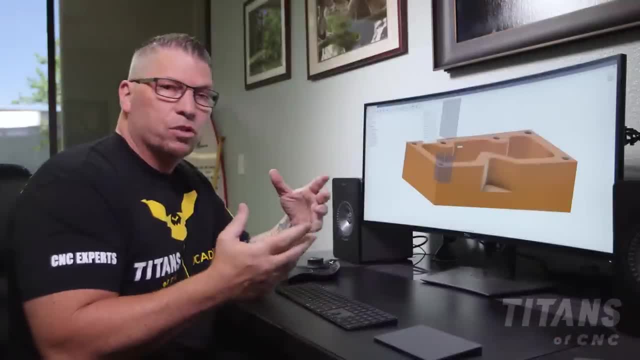 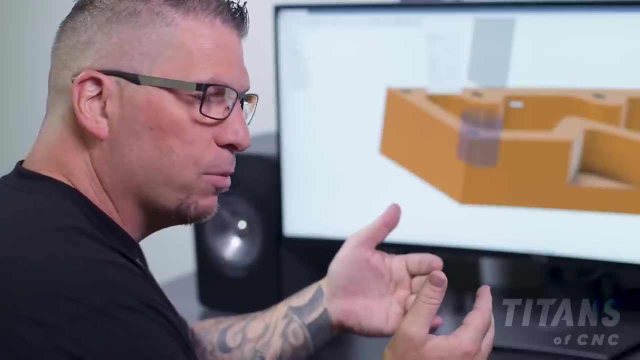 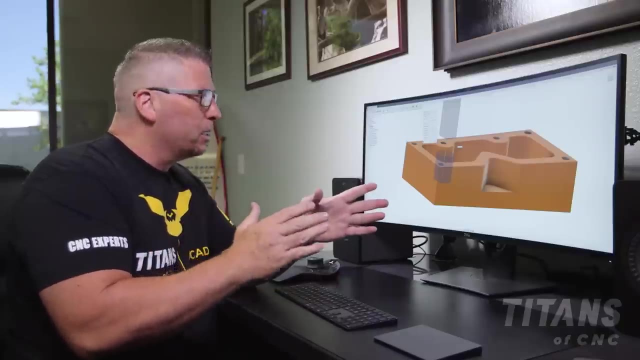 and just hogging out all that Inconel. All right, so now that we're ready to drill, let's look at the speed of the drill. So the recommended surface foot that I'm going to give you is about 70 to 130.. For the tutorial, I'm going to keep it on the low end, So I'm going. 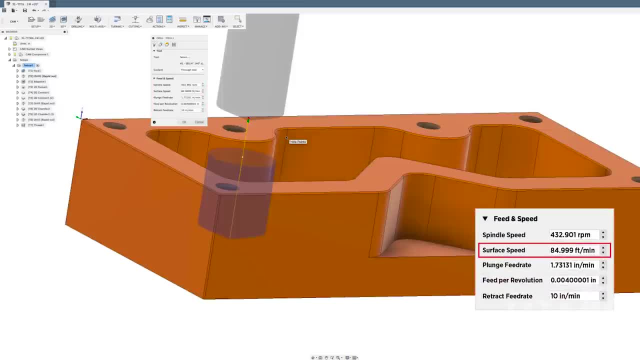 to keep it right at about 84 surface foot Nice and smooth Nice and safe and a perfect speed. And then, when it comes to the feed per revolution, I'd say that we're about four thousandths to six thousandths In this particular case. we're just putting it. 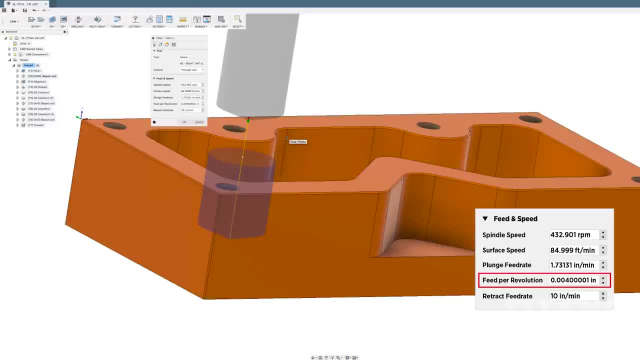 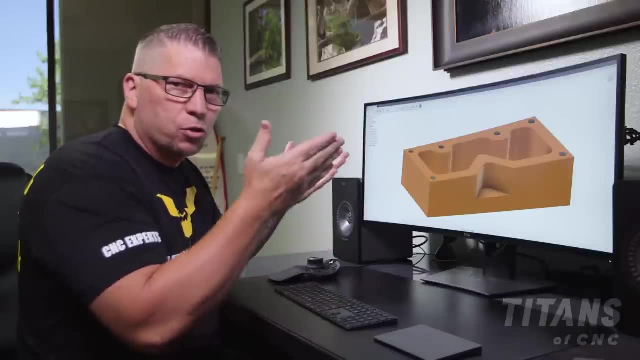 right at four thousandths to hug that bottom level, which will give us a perfect hole. So one of the things that I've done here is I don't actually know where the end mill is going to come down, but I know that it's going to rough this pocket. So what I did was I actually went to 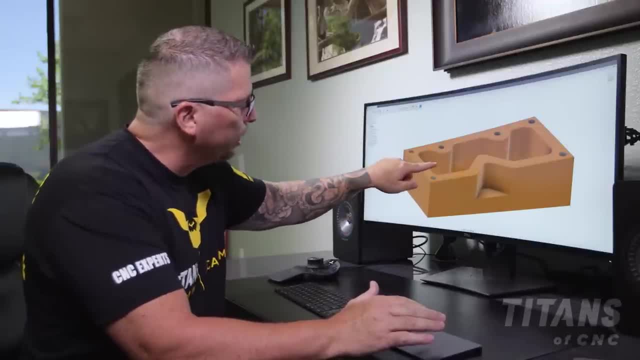 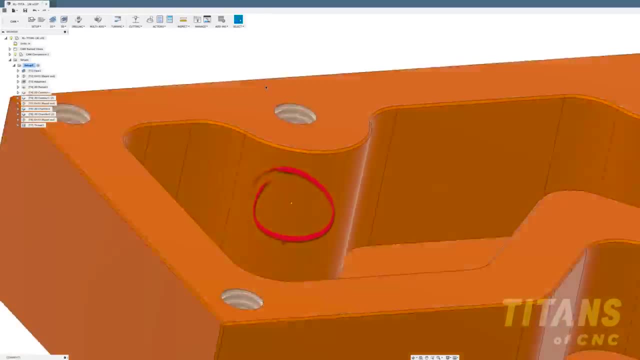 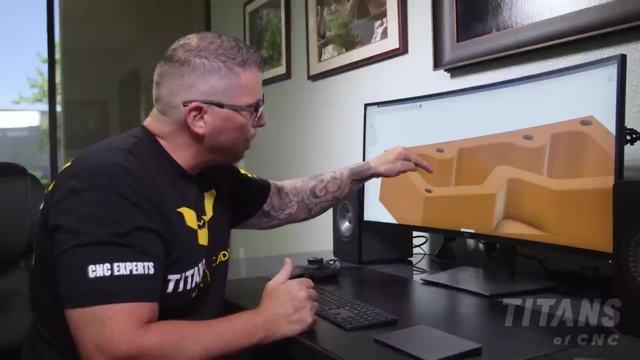 this surface and I actually drew myself a point. So that point right there. let me bring it up, This point right here. I basically just sketched it right there on that surface, right there, And then when I call up the drill location, I'm just going to hit that point right there and the drill will. 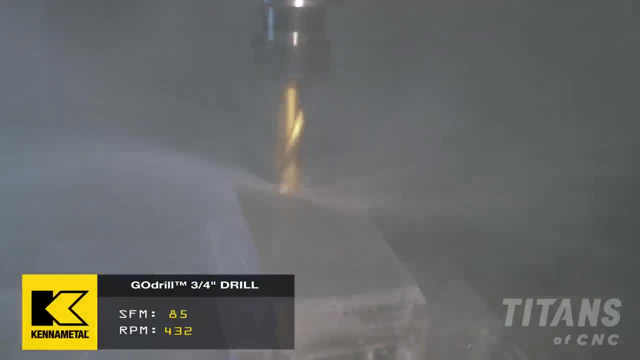 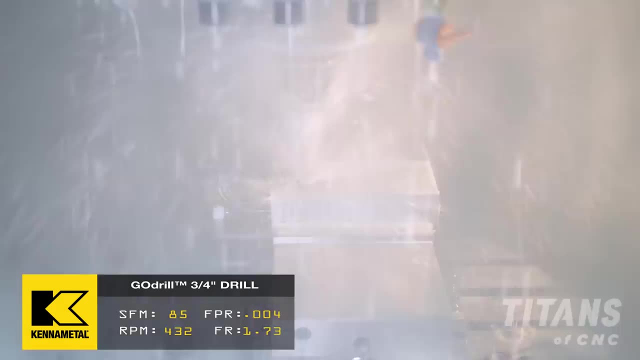 come down in that place And then when I go to do the pocket with tool three, I'll tell the tool that drill and it will automatically know to drop down at that exact location and start from there. Another thing that I'll point out is that this is a coolant through drill. This is a drill that 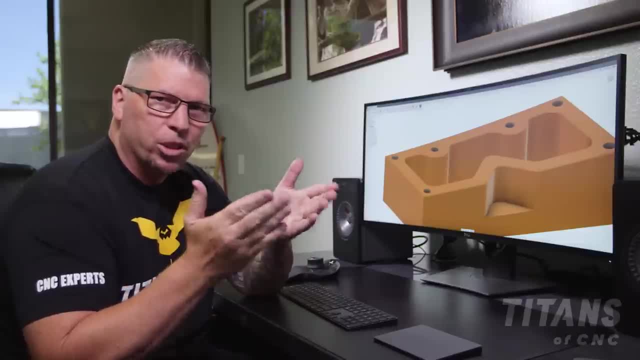 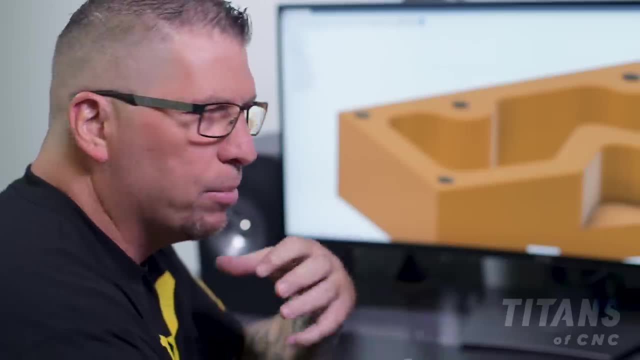 is specifically designed for hard materials and for getting the job done. So a lot of times when we're running aluminum, we're packing and we're just trying to get the material out in a hurry. In this case, we're simply going to grab the drill. 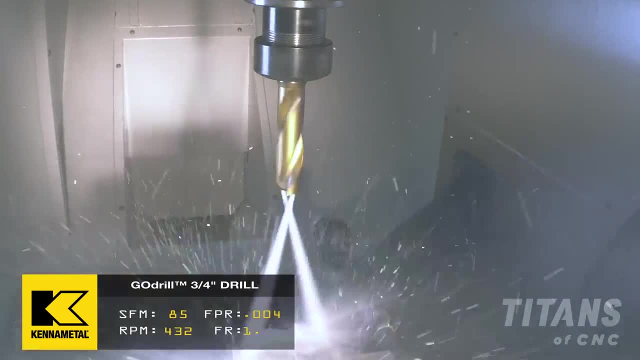 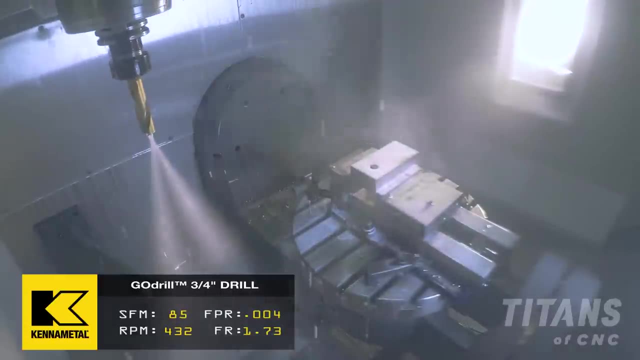 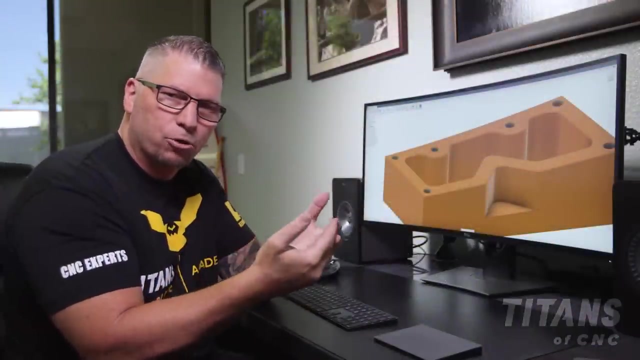 We're going to bring the drill down and then we're just going to drop full depth without pecking. Then we're going to come out and go get the next tool, Nice and simple, Even though it's Inconel. we don't have to peck because the coolant is actually flooding the front end of the drill. 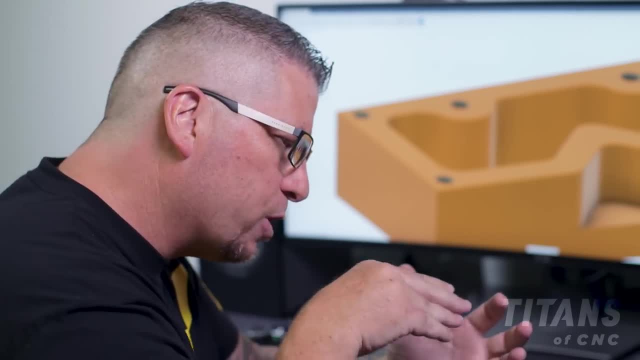 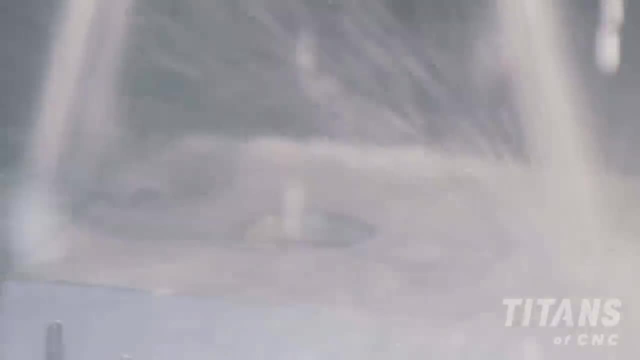 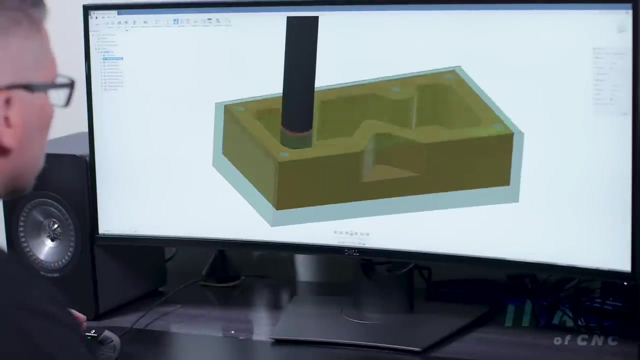 And the drill is designed in such a way that, as it drills down, it's breaking that chip and the chips are just flowing out of the hole, All right. so now that we've pre-drilled the pocket, I'm going to go to an end mill to rough. 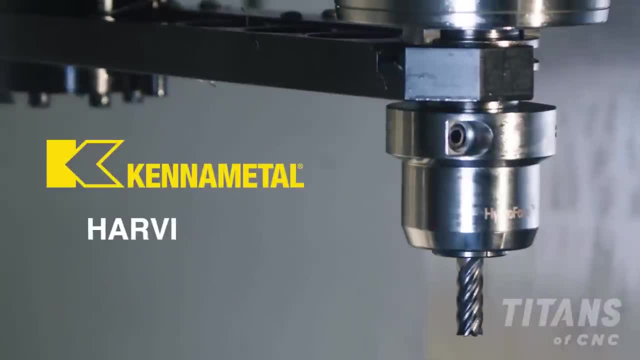 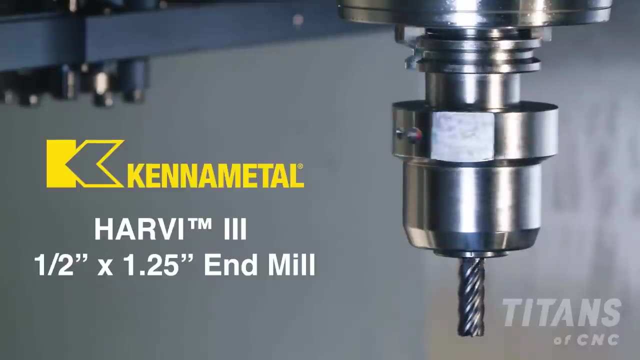 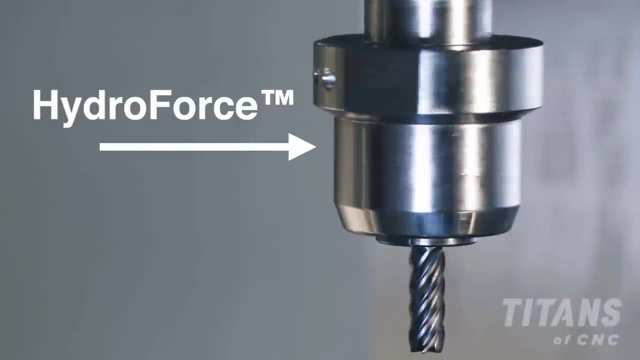 the pocket out and rough out the outside. I'm going to go to the Harvey 3 and it is a beast of a tool. My team actually nicknamed it. We called it the zombie cutter. This thing was dead and it just kept coming. All right, so now let's talk surface foot. When I'm in titanium, we're peripheral. 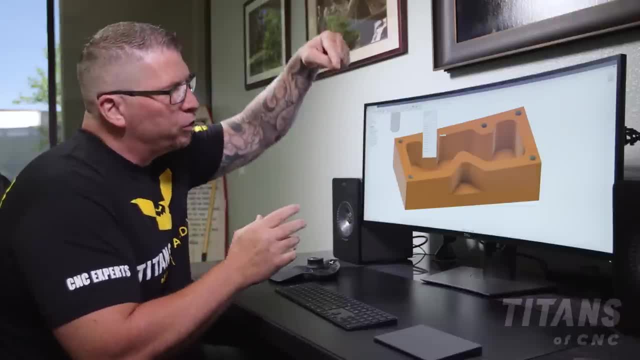 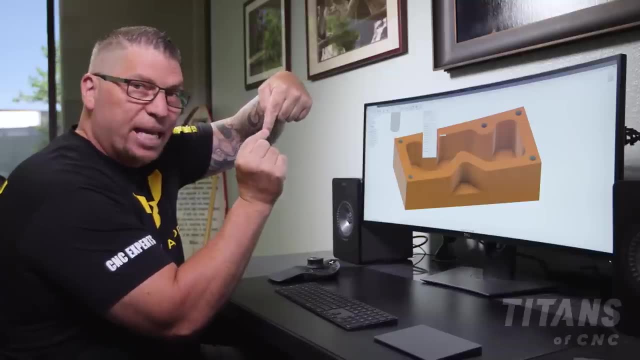 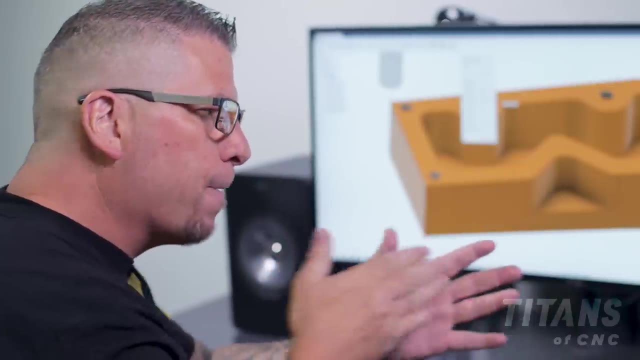 right. So the old style of machining: you actually drop down and you're only using the tip of the cutter. The cutter's flexing and you're taking a big cut with the tip right. But now we're creating tool pads that, instead of plunging off a dock, they actually ramp into the material taking. 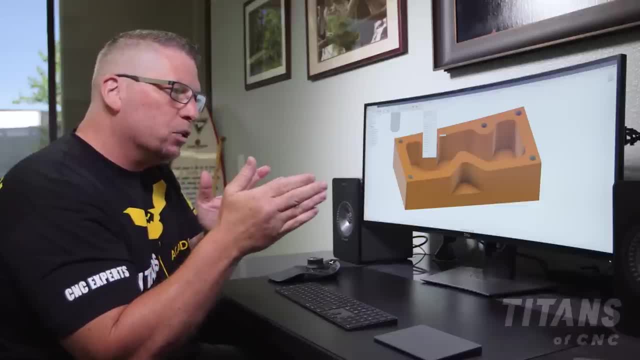 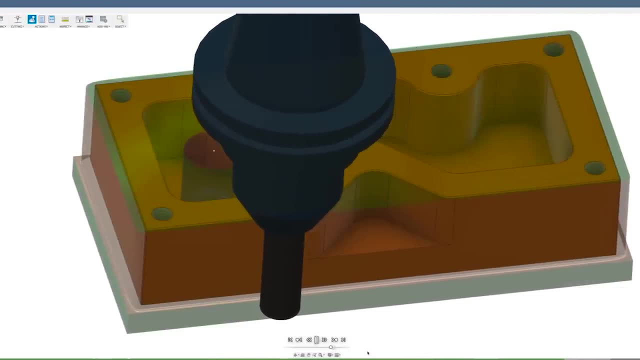 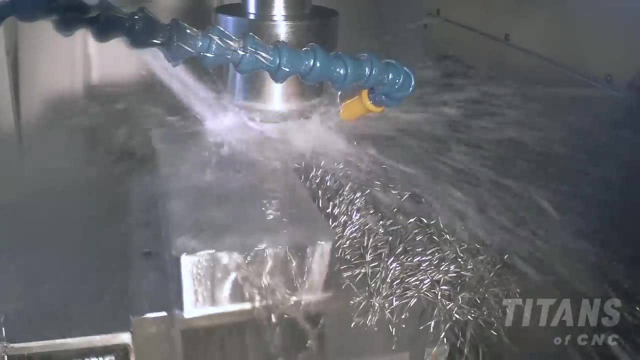 the pressure off And we take a smaller radial, but we drop full depth, utilizing the entire flute length, which brings stability and rigidity and allows us to go much faster. So in titanium, if you look in the machinist's handbook, you'll see 175 surface foot as a standard. But in Inconel, 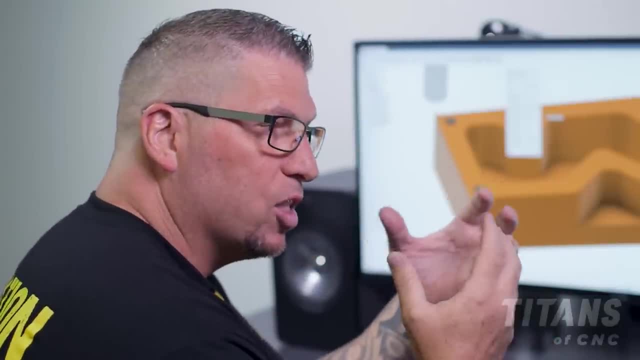 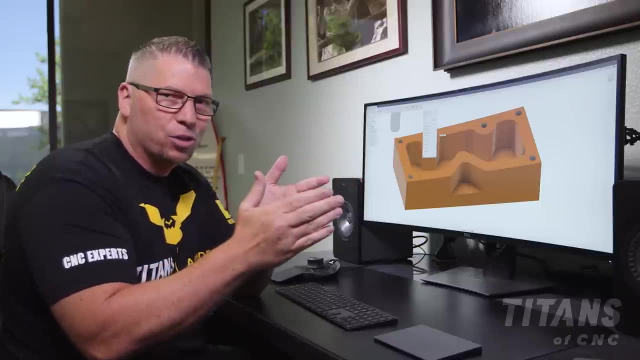 it's another story, right, Inconel is much harder than titanium, So the surface foot is on the low end. So, instead of 175, you're talking, you know, 50 to 100 surface foot, right. However, because of 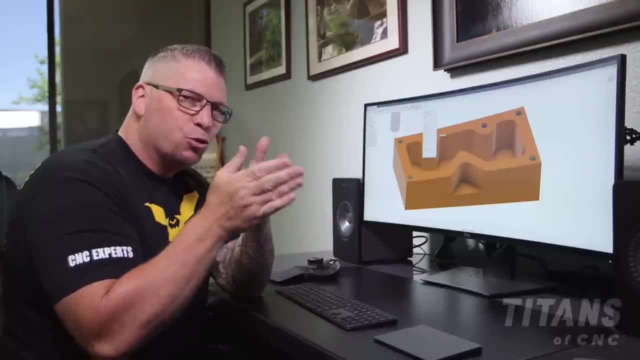 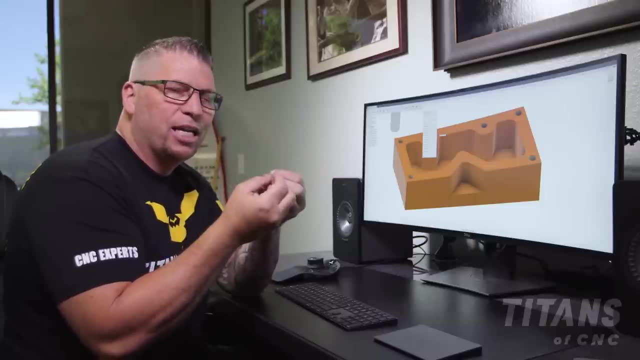 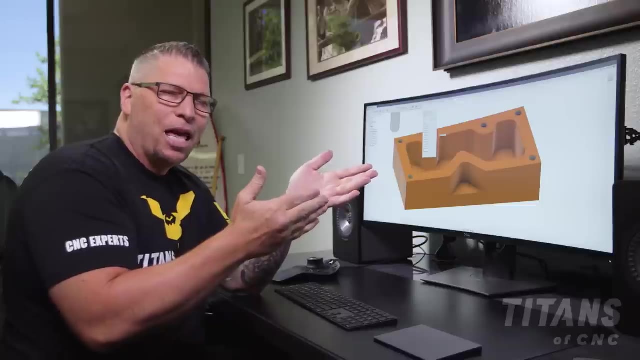 the tool pass, that we're using the rigidity in tool, that we're getting the coolant, that we're using all of the variables put together. we actually run from 200 to 400 surface foot in Inconel And we do it in a consistent manner over a long period of time. okay, It's not just. 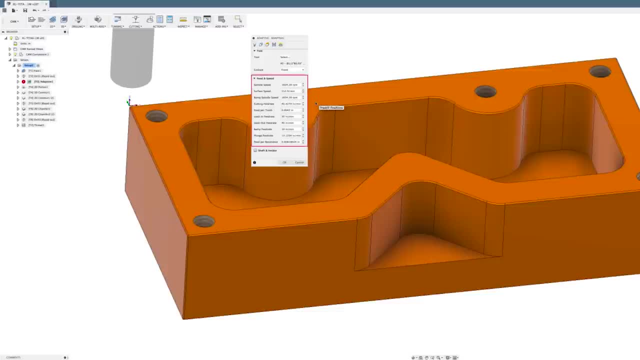 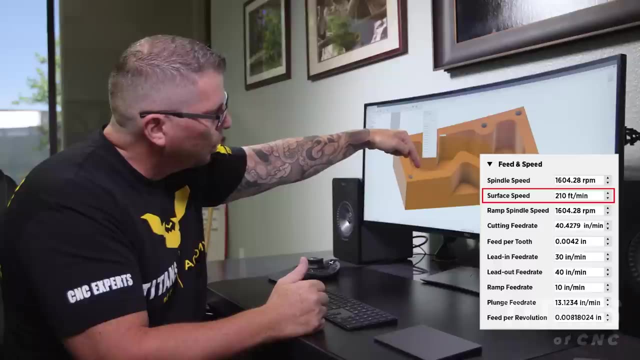 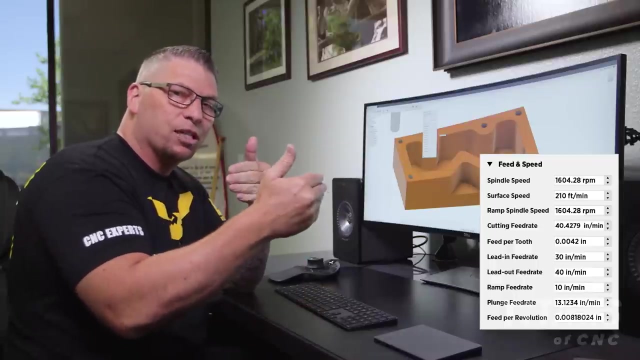 something that we're practicing with. So in this specific application we're going to run at 210 surface foot. okay, We're going to keep it on the low end On the inside and the outside we're going to drop all the way to the bottom. Now our radial depth of cut, So we're full depth. So if 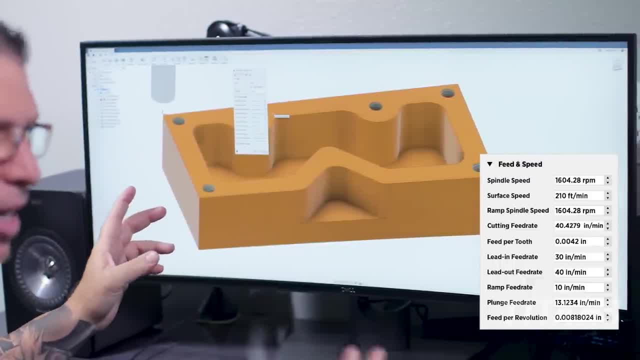 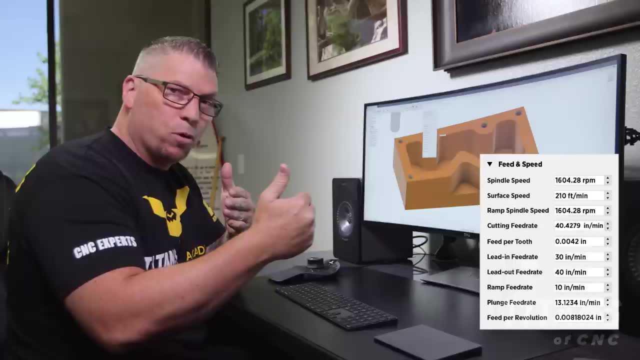 you look at the outside, you're probably at two and a half times diameter. That's deep Now radially. instead of taking a big step over, we're actually going to take a 4% of diameter step over And then 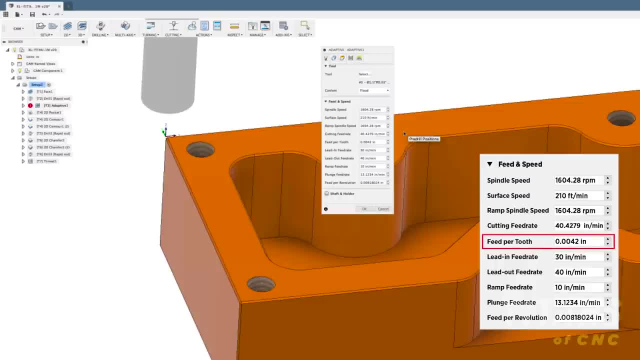 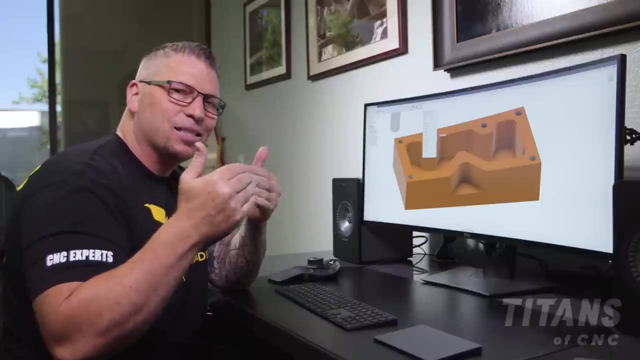 we're going to put our feed per tooth at 0.0042,, which is going to give us a feed rate of 40 inches per minute, which is incredibly fast for Inconel, And yet it's safe and will be consistent in the 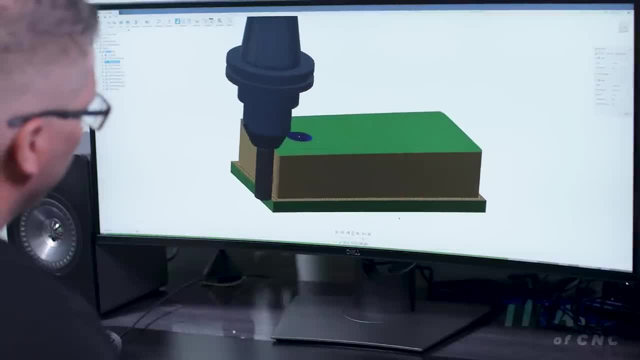 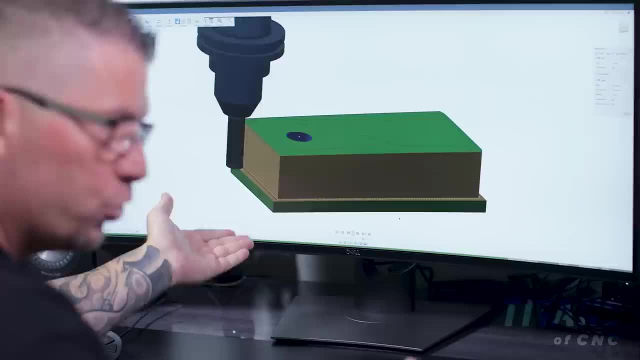 cut. So basically, what you see is the end mill is actually taking about 20 thousandths per cut, but your 1.2 inches is going to be a little too deep, right? So it's just going around and cutting all the. 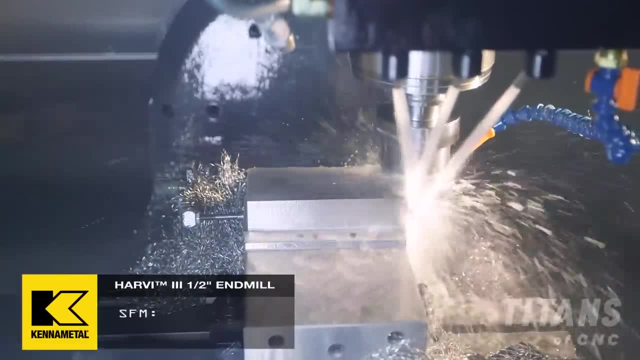 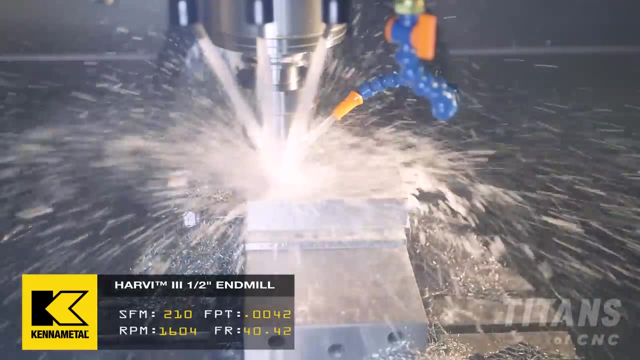 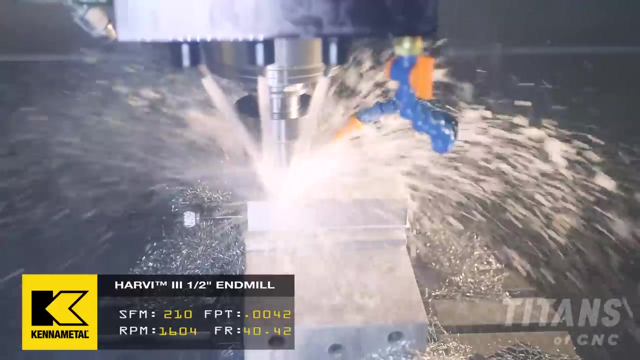 excess material. We actually had more material on the outsides on X than we did on Y, and that's why it's going and finishing everything Now. it dropped into the pre-drilled hole and now it's peripheral milling And now it's actually cutting material. 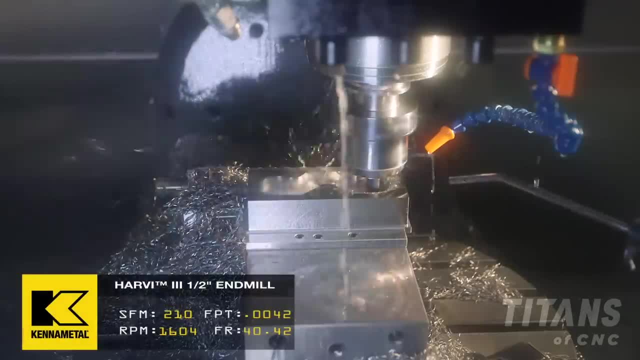 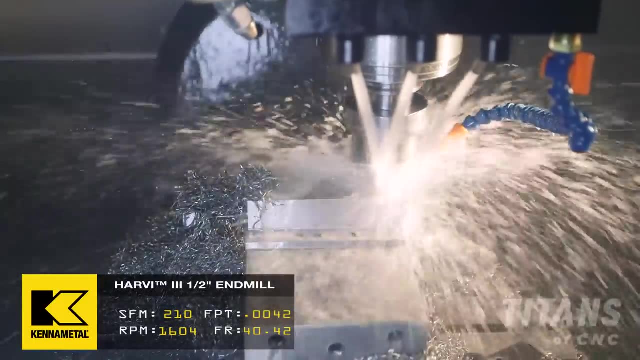 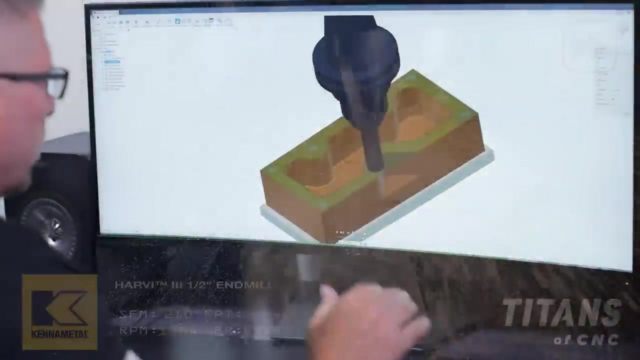 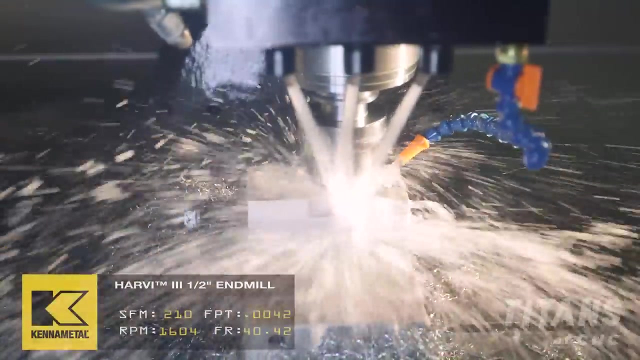 Now it's going to come over there and rip out this section. 0.011, 0.012 000 000, 300, 0.033, 400 500, 8 Qi 100. 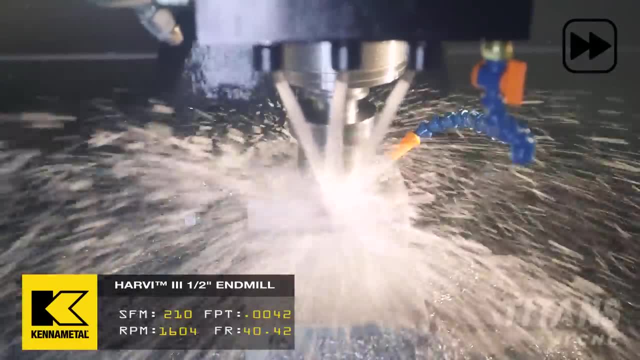 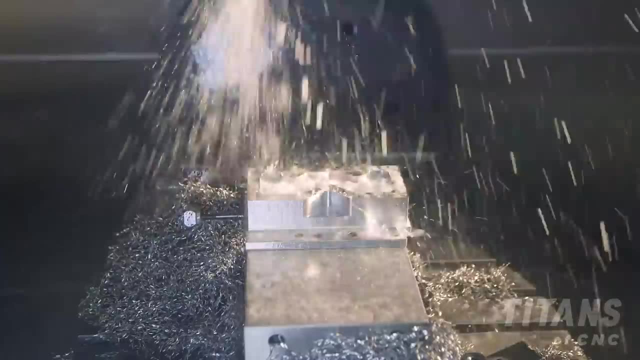 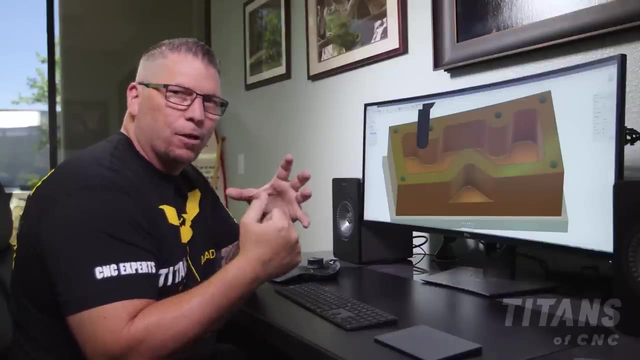 All right. so everything's been roughed and we left five thousandths on every surface. So now we're going to come back and we're going to kiss it. All right so a Harvey 3 end mill roughing Inconel. It's going to get dull, no matter what. It'll keep going and sometimes go for hours. but 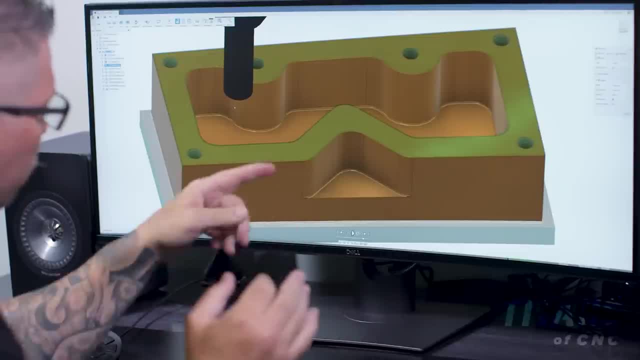 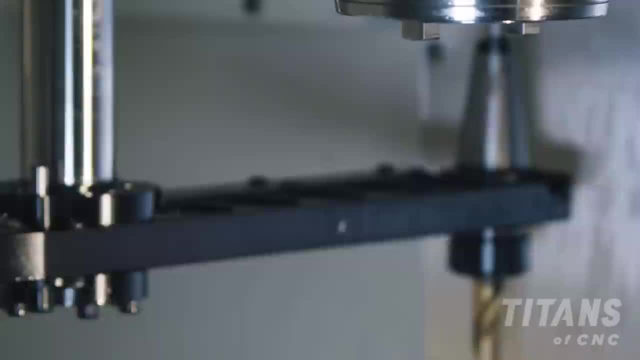 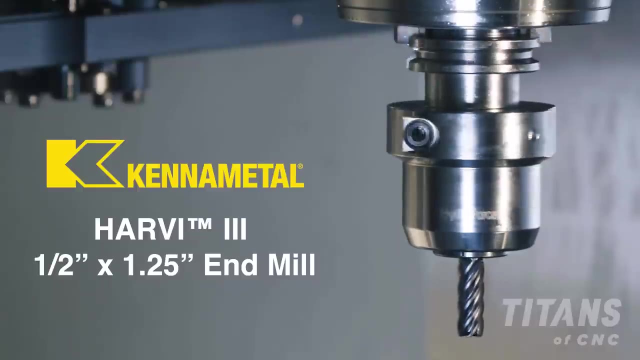 since we're looking for a perfect surface finish on these walls, I'm simply going to use a different tool to come back and kiss the side. So now we're using a different Harvey 3 end mill to actually finish the part. Now, with tool four, we're going to drop into where we previously roughed and we're 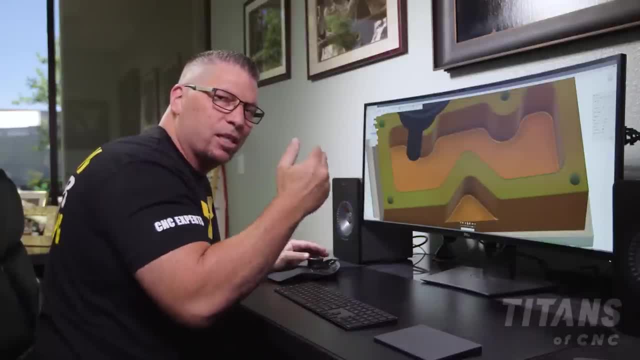 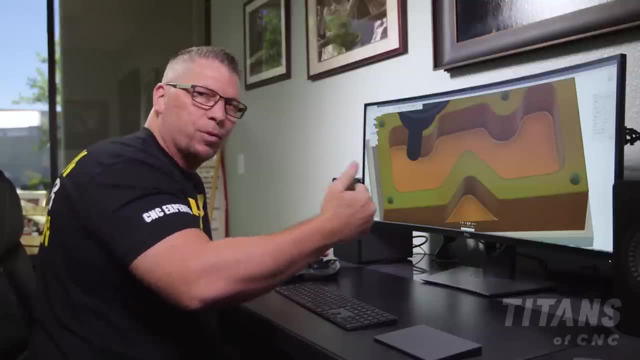 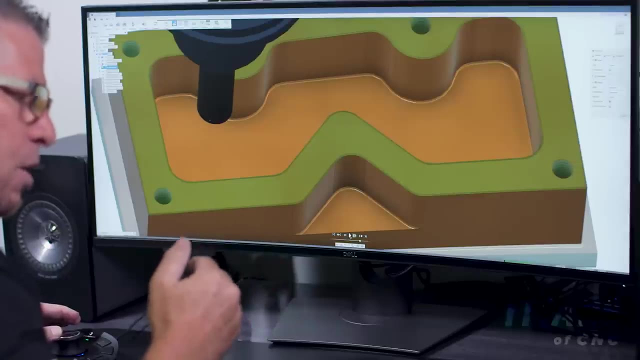 just going to kiss the bottom. But guess what, instead of a twenty thousand step over, my step overs are much greater now, Because I don't have all of that material to cut through. I'm only cutting the bottom surface and I just want it to be beautiful, Right? so I don't want all those lines. So now, instead of a twenty, 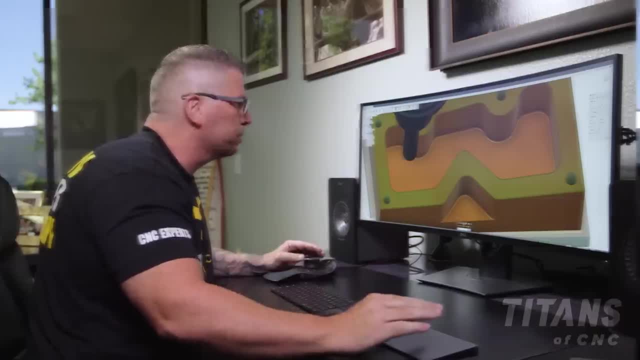 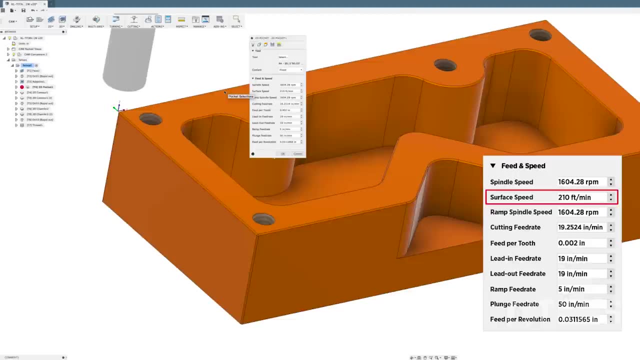 thousand step over. I actually have a greater step over. All right. so when it comes to the speeds and feeds on the surface footage it's exactly the same, Two hundred and ten SFM, But the chip load, the feed rate per that revolution I've dropped in half. 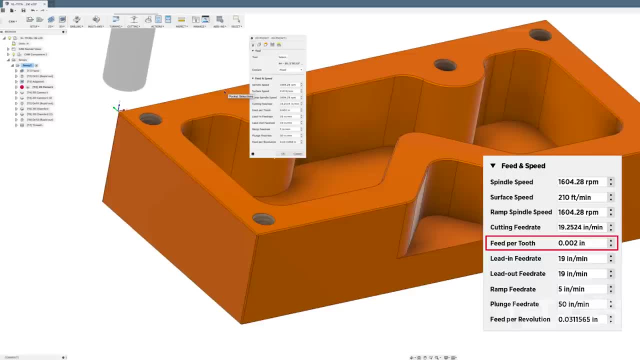 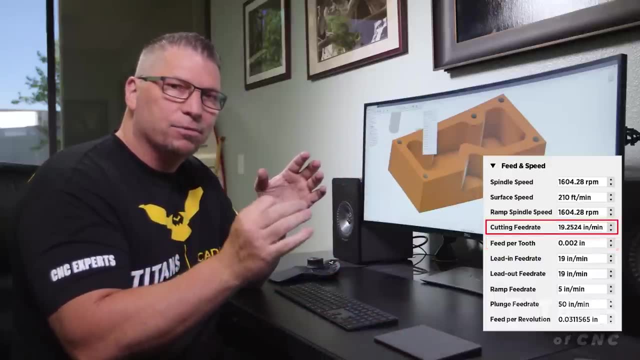 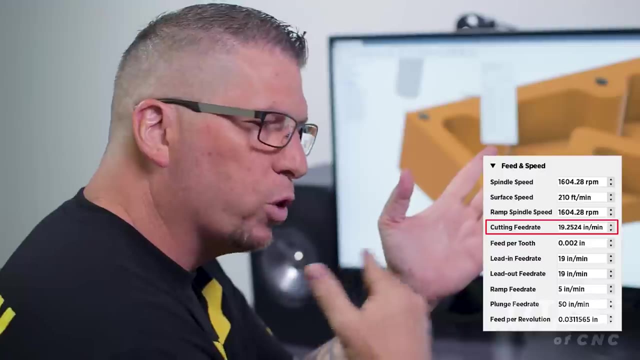 So instead of being four thousandths, we're at two thousandths chip load. So point zero, zero two, which gives us a cutting feed rate of 19 inches per minute. All right, so we already know, with the current RPMs at 40 inches a minute, it can rough all day. Boom, boom, boom. right, But now all we've 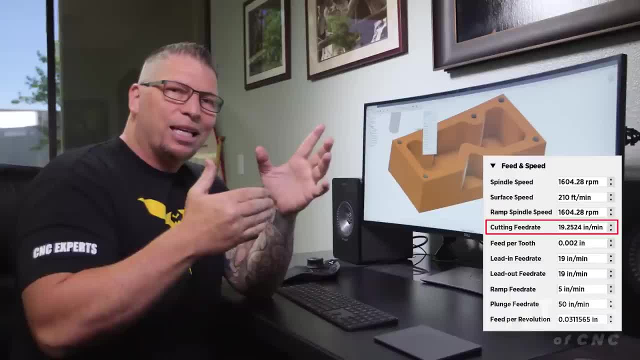 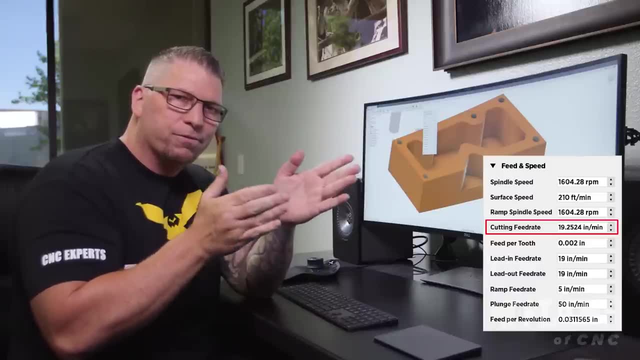 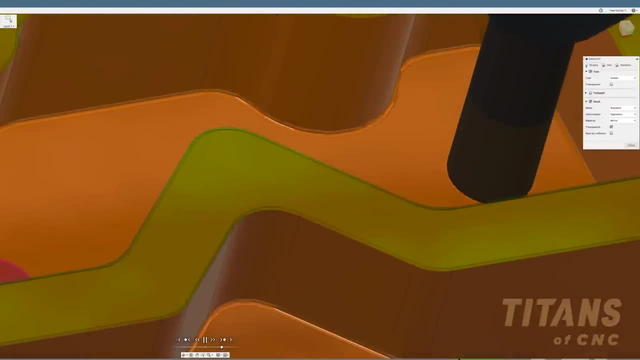 done is, taken the feed rate, dropped it in half So that we can allow the chip load to come through And allow those cutters to work and give us a perfect surface finish. So tool comes down ramps into the bottom, comes over here, drops down ramps into the bottom. 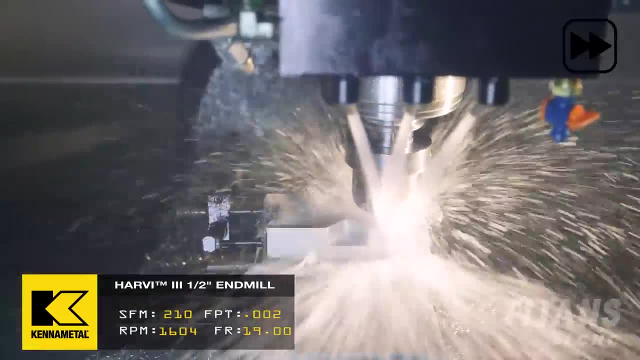 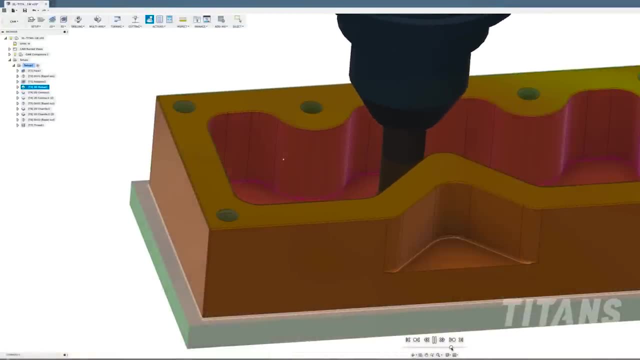 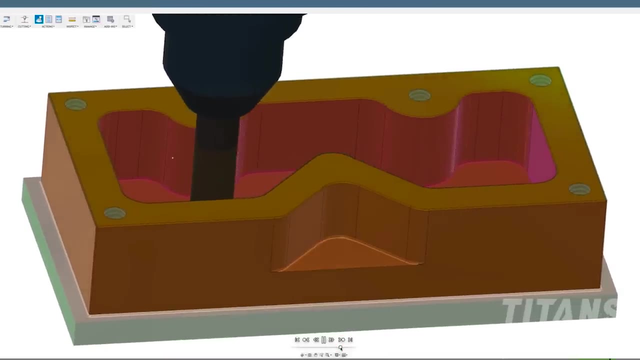 Because the tool is pretty long and taking the entire wall and I want to have a perfect finish. I'm actually finishing the inside wall and then I'm going to do a spring pass just to catch any of the deflection Right. so the tool with the pressure is going to want to deflect a little bit, Which is going to make it so. 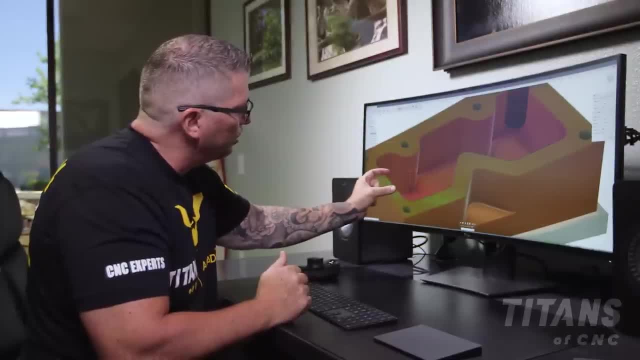 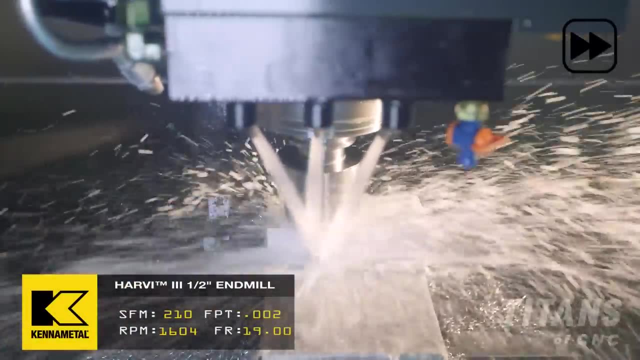 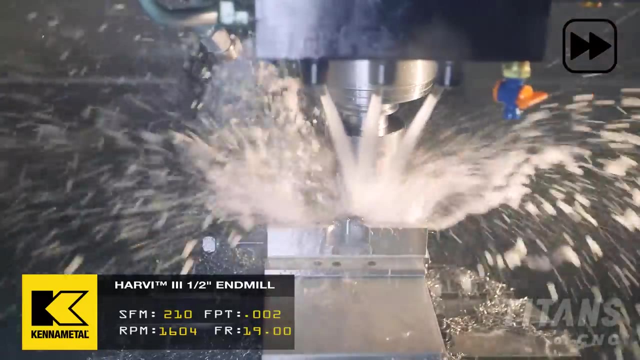 you might have a perfect tolerance up here, but the bottom might be a little bit small because the tool deflected outwards. All right, so now I'm coming on the outside. I'm simply kissing the outside, doing a 2D contour All the way around. it Flip around to the back, Just doing a 2D contour all the way around. 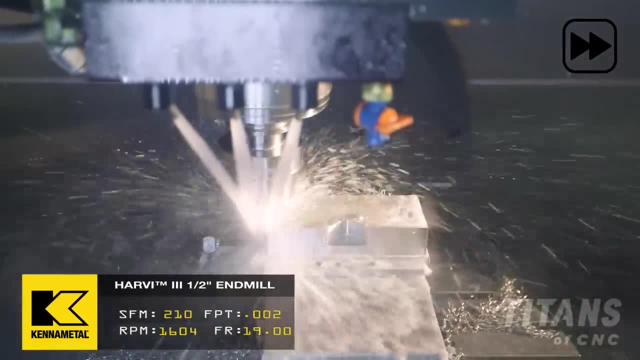 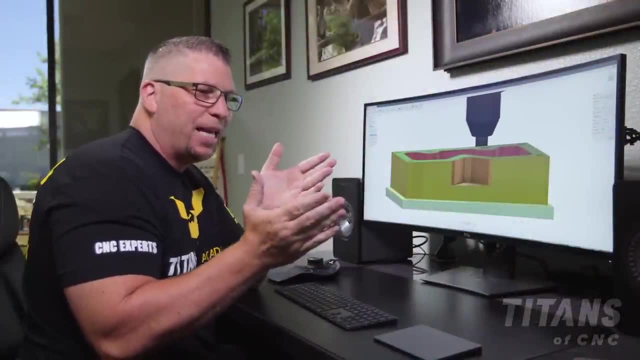 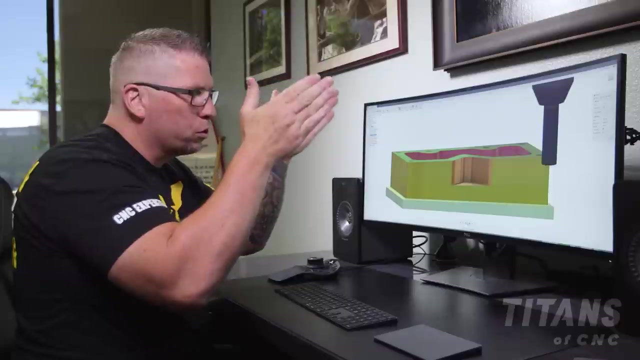 I'm taking a five thousandths finish pass. There's my spring pass, So I'm not cutting extra material, I'm just picking up anything that was left Because the tool deflected, Because I want those walls to be perfect And perpendicular to that top surface. 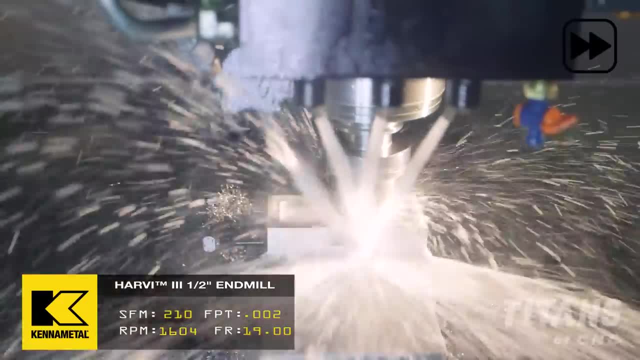 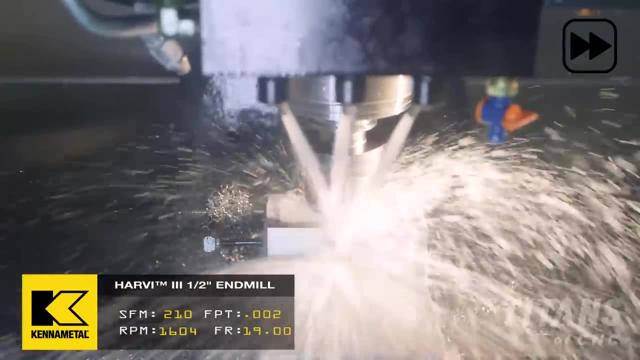 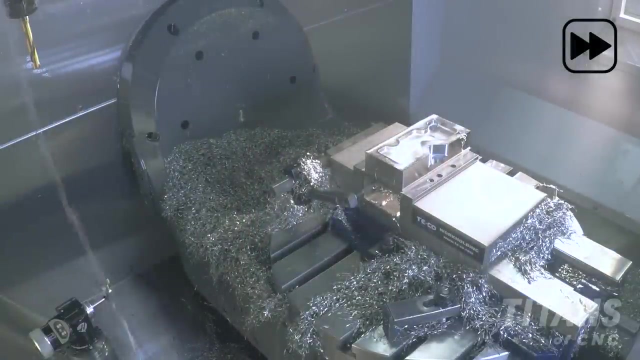 Took my first cut right there, Took my second cut to finish that surface, All right. so now we have come back and actually done all our finish passes To kiss all the surfaces and the bottom of the pocket To make it all perfect and to size. 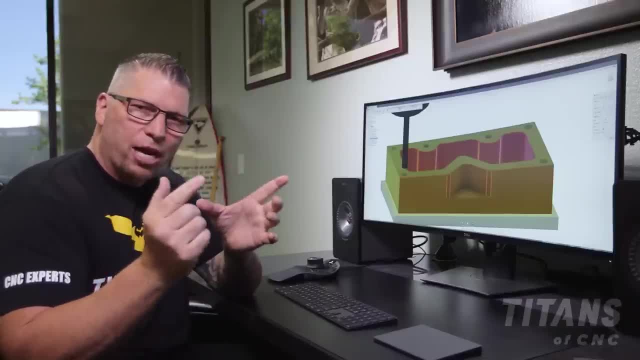 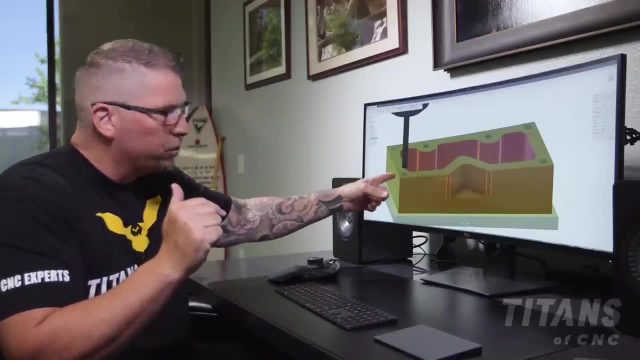 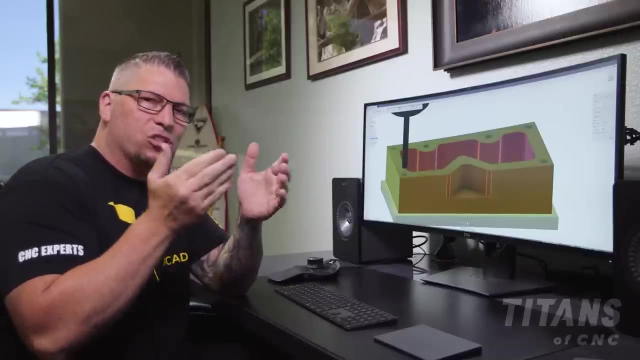 If this was aluminum I might come back with a chamfer mill now and actually chamfer all those edges And actually spot drill where my threads are going to be. But this is Inconel. So I have a different approach because I don't want to send a tip of a center drill or a chamfer mill straight into the Inconel. 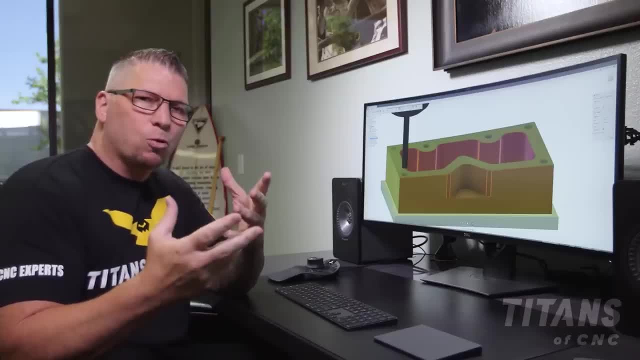 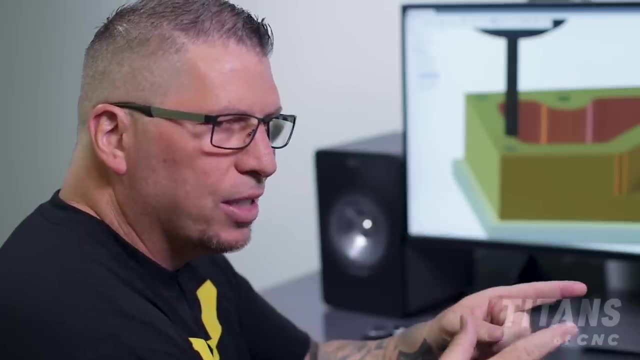 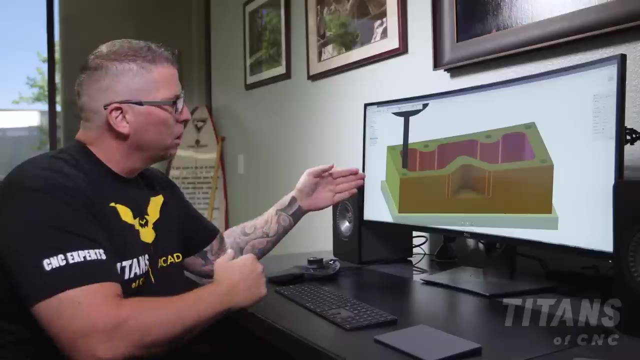 It might handle for a while, but it will wear out. So, strategically, knowing that the go drill is self centering, I'm actually going to drill first and then chamfer the outside afterwards. So this is a go drill, just like the three quarter inch. 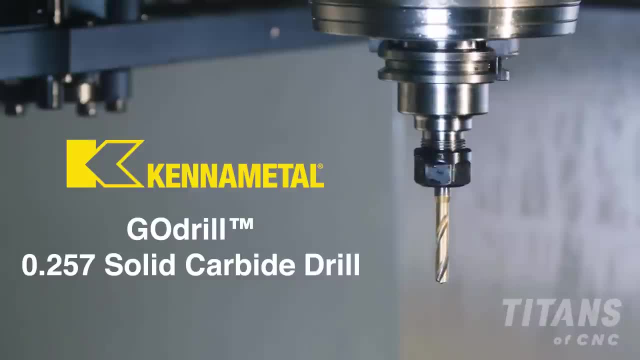 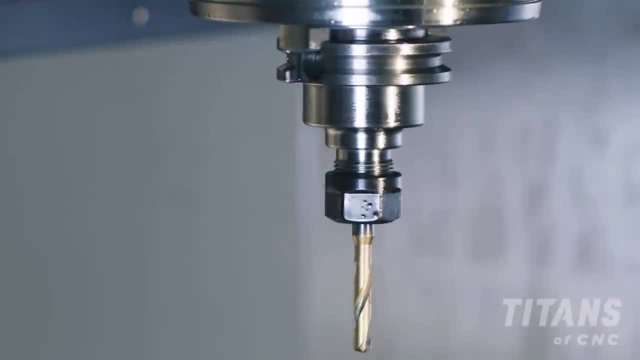 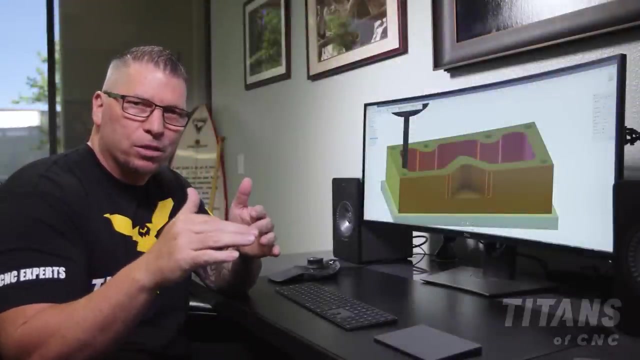 But this one has a diameter of .257.. Which is the minor ID for a 5, sixteenths 18 thread, Which we will then come back and thread mill. But now we're going to pre drill the ID of that thread. 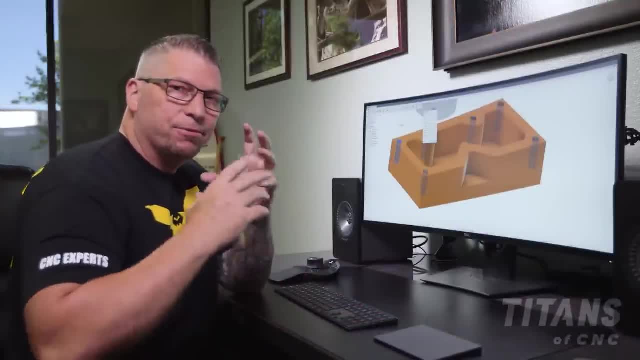 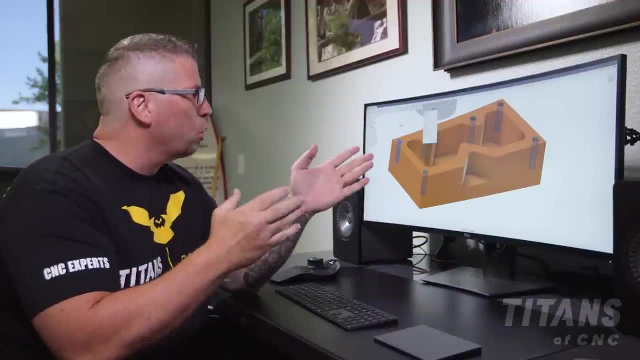 All right, so the speeds and feeds. Remember what the surface footage was. It was 70 to 130 in Inconel. So we're going 85. It comes up just a little bit. It's not under 85. But it's basically 85 SFM. 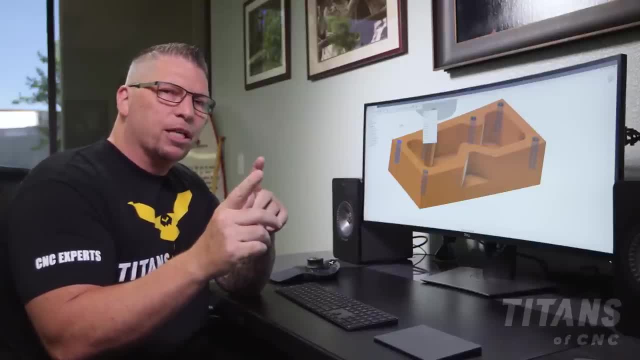 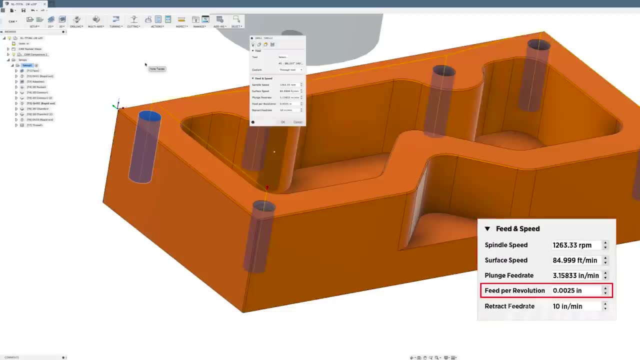 All right, The chip load on the smaller is going to change a little bit. Okay, So it's a little bit more aggressive for the bigger tools. On the smaller drills, I like my feed per revolution to be about two thousandths to three thousandths. 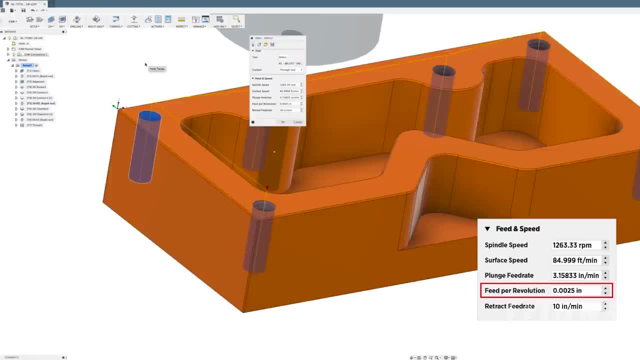 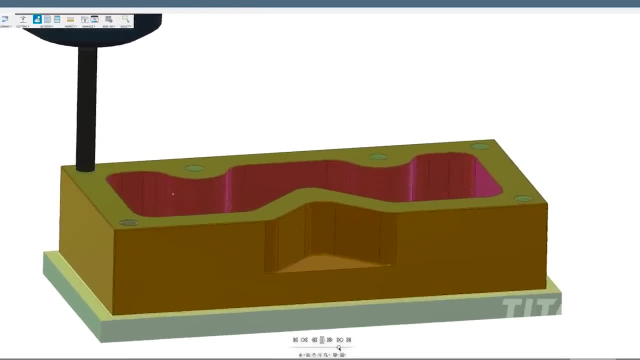 All right. So let's just split it in the middle and go .0025.. And then we're just going to drill straight down, Come out, Go to the next hole And boom, And we will get a consistently perfect series of holes. 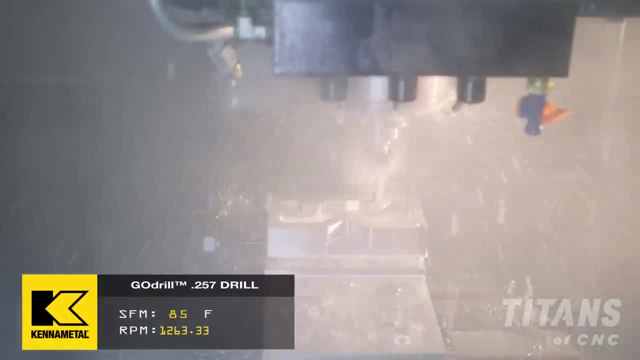 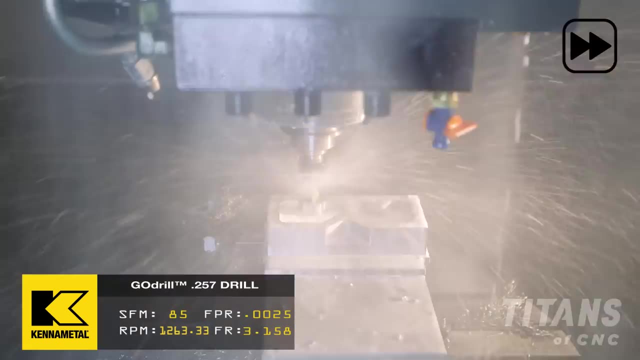 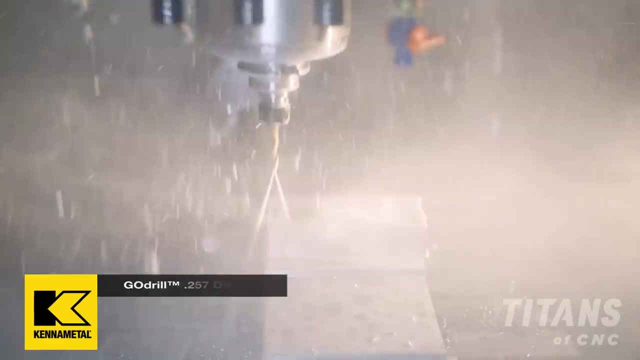 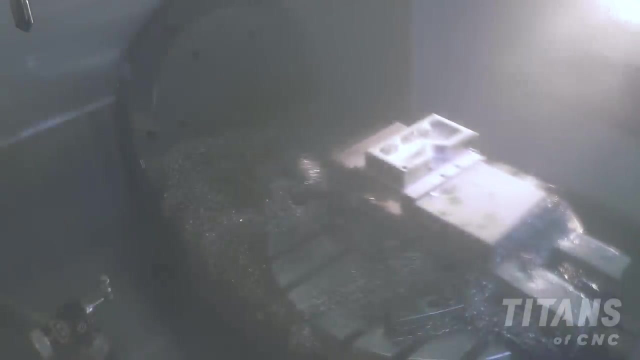 Same thing. There's no peck. I'm drilling straight down, The coolant is blasting from the tip And it's just boom, boom, boom, All right. So now that we're finished drilling The .257 diameter hole, We're going to actually bring in our chamfer. 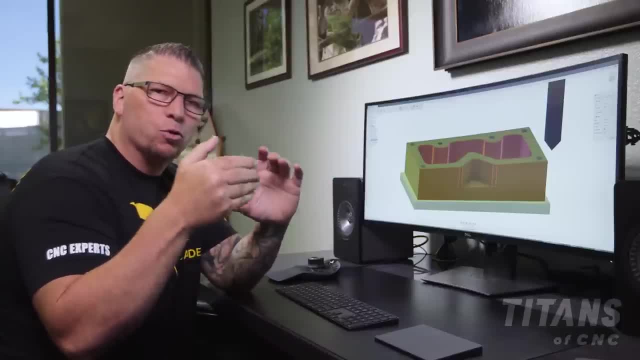 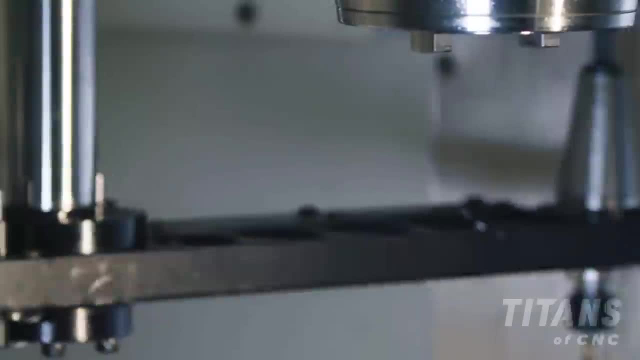 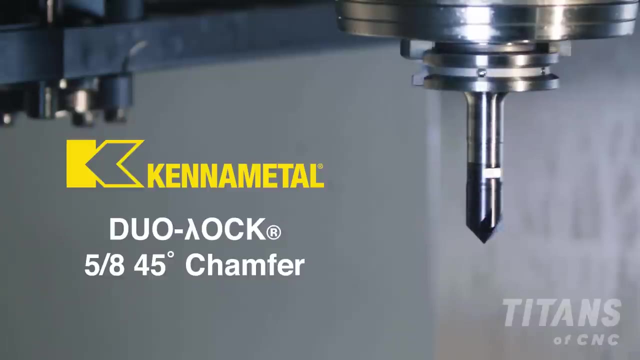 And we're going to actually spot those holes to create the chamfer for the .516, .18 thread. All right, So tool six is going to be a .58 six flute chamfer mill at an included angle of 90 degrees. One of my favorite products that Kenna Metal has is the duo lock system. 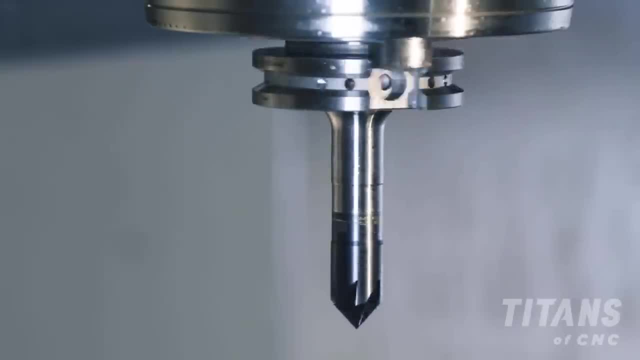 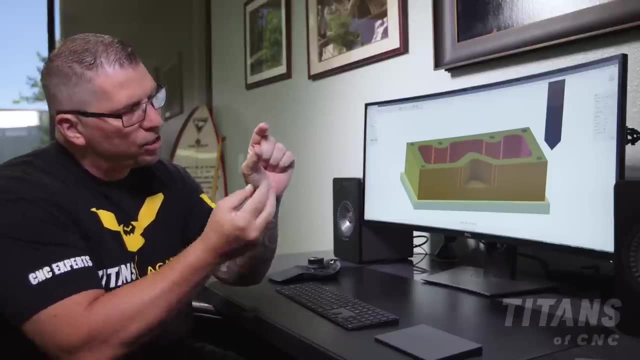 It's a way to save on carbide, All right. So when you have end mills, they literally, instead of having this much carbide, they give you just the end mill and actually put a tip on it that actually screws into a body, Right. 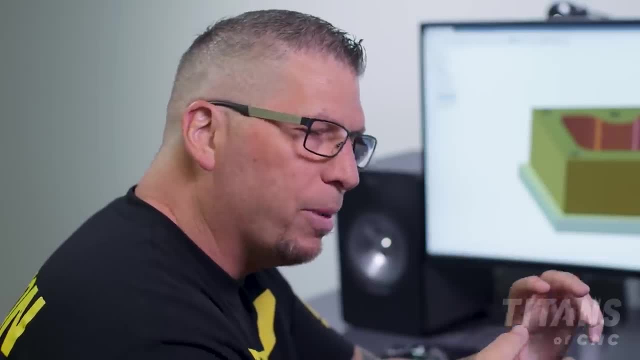 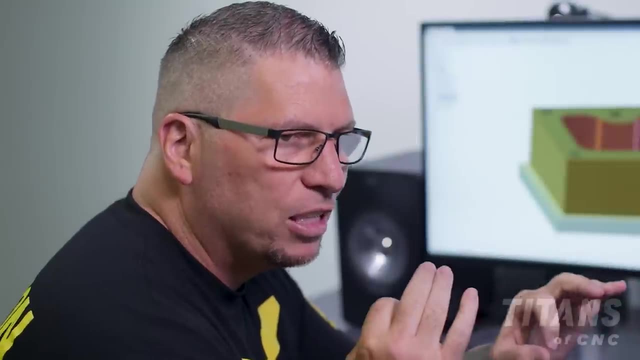 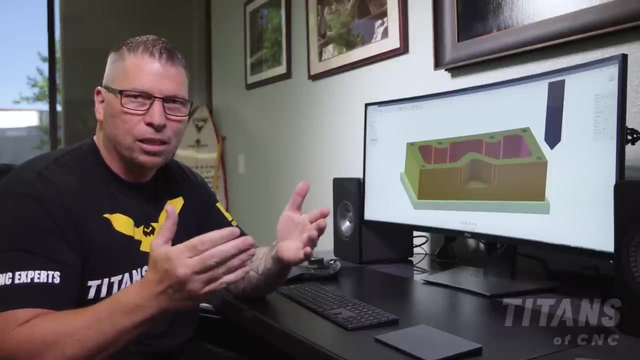 So it connects And then when the end mill wears out, you basically unscrew it, Put another insert in, Screw it back, Lock it. It locks perfectly in place And you just keep running And when you're running production. This saves huge money because you don't have to pay for all that carbide. 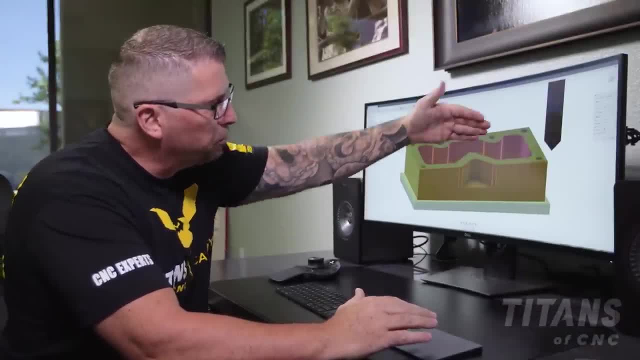 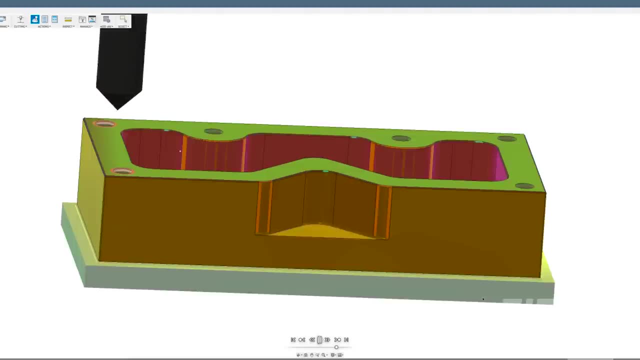 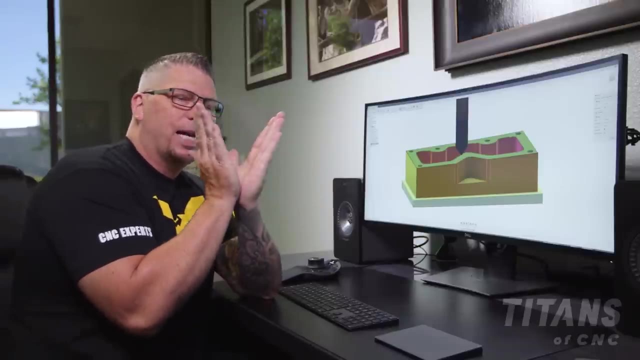 So now that we have the holes already in place, We're simply going to drop down and chamfer around the hole to a diameter that's approximately about 10% of the overall thread diameter. We're looking at a chamfer mill. We're talking a 90 degree included angle. 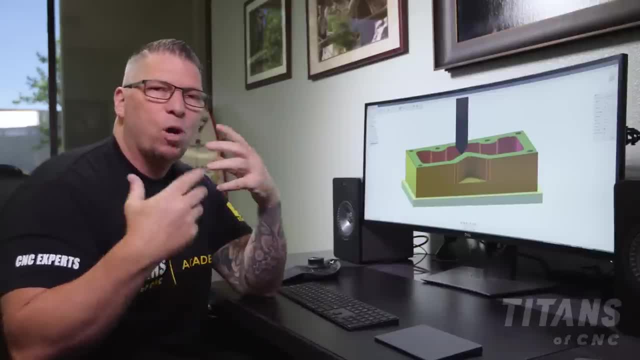 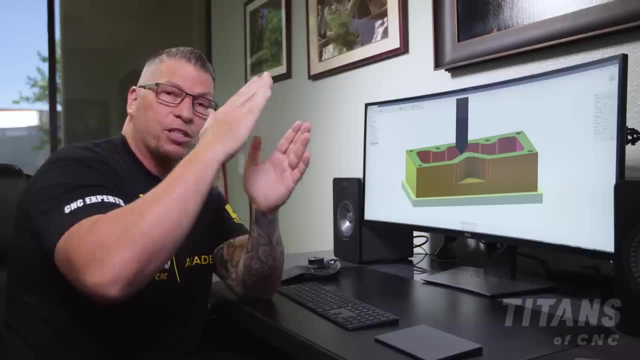 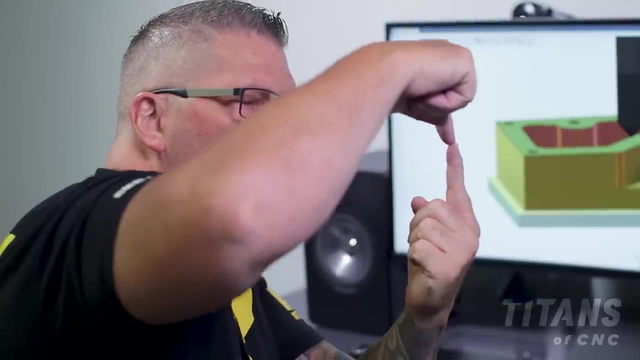 So each side is 45. Okay, That's why it's popular in machining, Especially manual machining, Because it's easy to calculate. If I have a 45 degree angle, all I have to do to calculate it when actually creating a chamfer is go edge to edge. 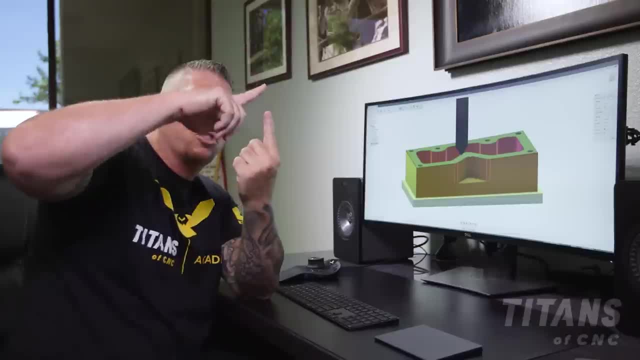 And basically I can just go. okay, I want to chamfer this edge 5 thousandths. All I would have to do is go 100 thousandths off, 100 thousandths down And then an additional 5 thousandths, Because it's a 45 degree, it's equal. 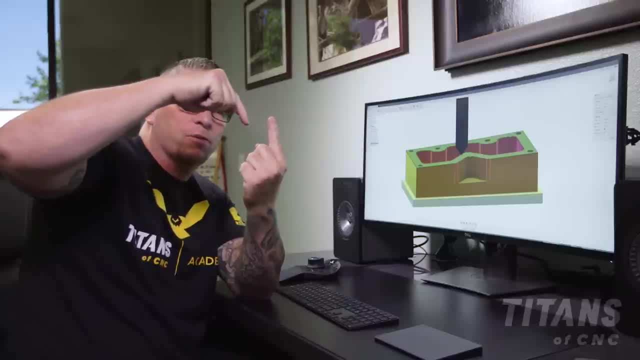 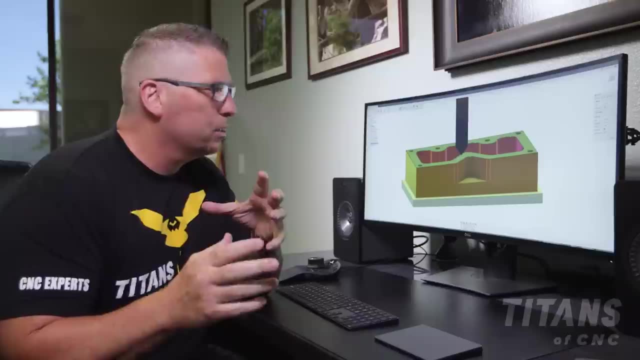 So 50 over 50 down, 100 over 100 down Creates edge to edge. Anything beyond that is the chamfer Alright. So when it comes to Inconel, I'm actually I have a 5 eighths. 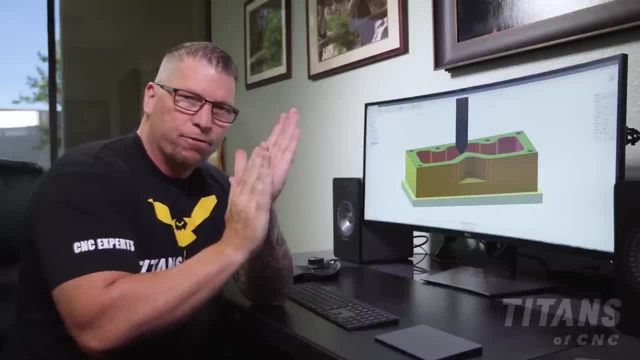 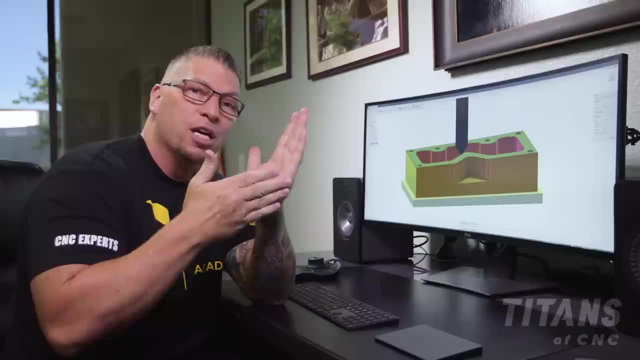 So in aluminum I might say it's a 100 thousandths and it's 50 off and 50 down Right. And if I wanted to do a 10 thousandths chamfer I would just go 60 down Right. So it's 50 off. 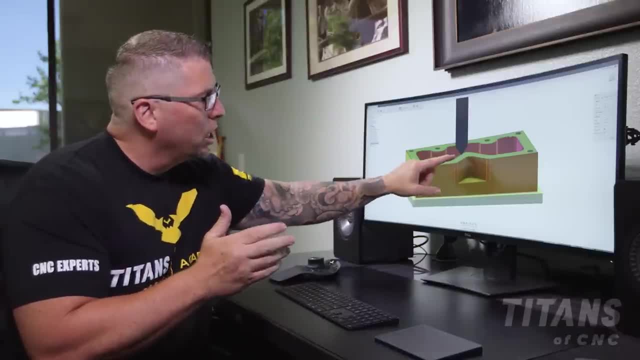 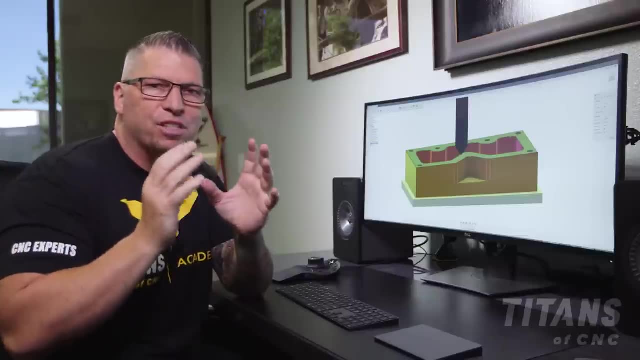 60 down, But because it's Inconel, I want to use the flute higher up And I actually want to give it some room to actually cut because I have 6 flutes. Okay, So on the top surface, I'm basically going to hit right kind of in the center of the flute. 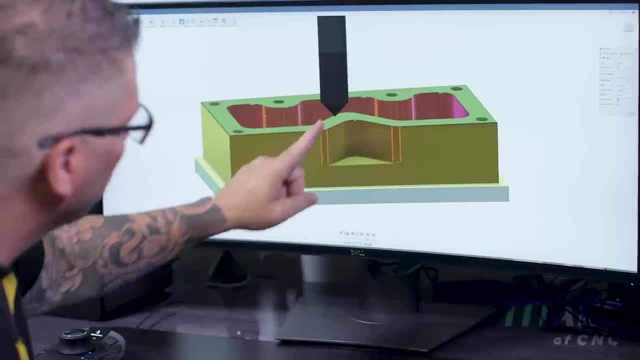 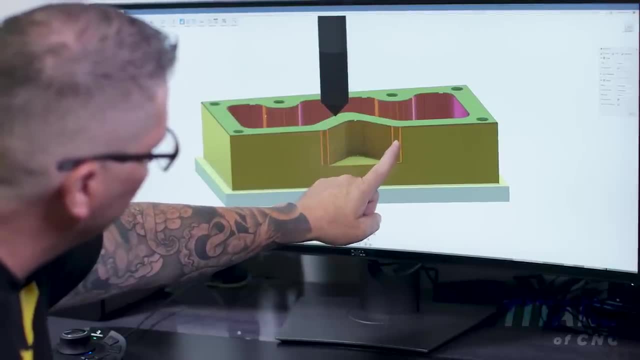 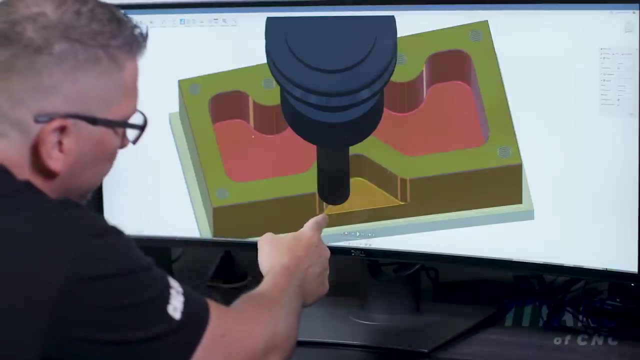 Alright, That's good, But On the bottom surface, The closer I get to the tip, The farther the tool is going to have to be away from this surface Right. So when you look at this surface, If I'm close to the tip, 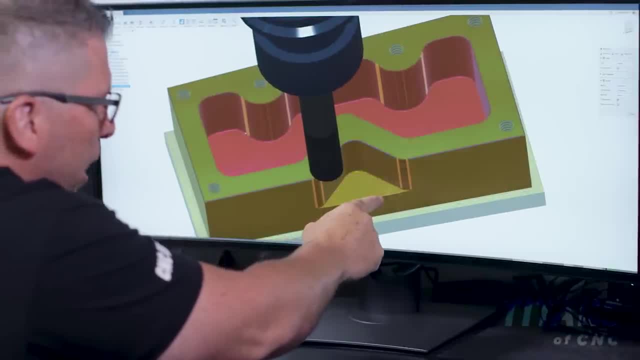 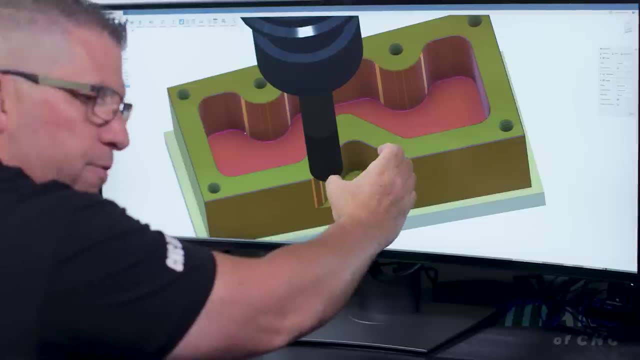 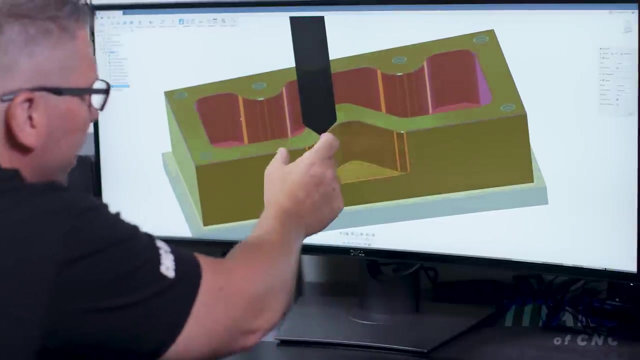 I'd have to pull my tool away from that surface, And that means that the chamfer would be only over here Because the tool was away from the surface. So what I'm going to do is actually call it a larger diameter. So the software takes the tool. 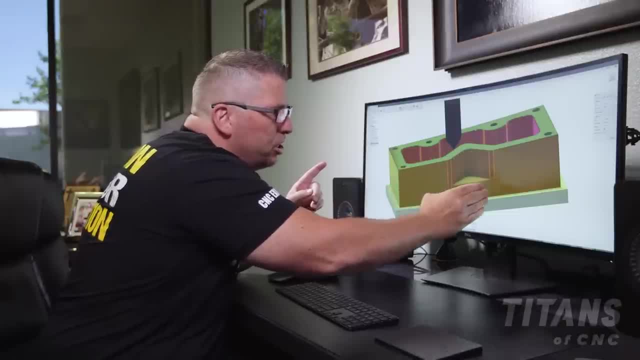 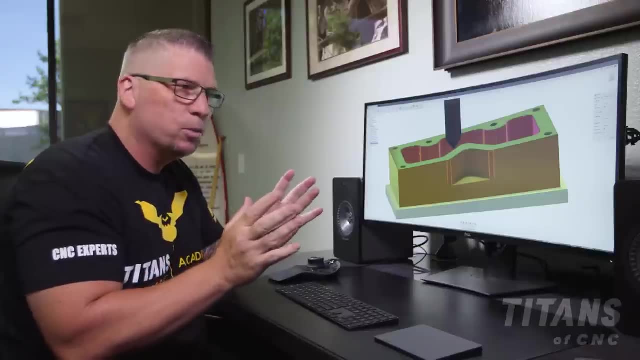 And puts it right up against the wall, But deeper, So I can get my chamfer all the way over here. So just like a little trick, Right? So if you're running aluminum, That's one thing, If you're running on the top. 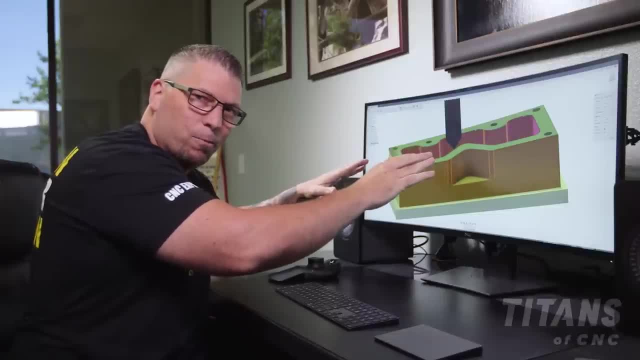 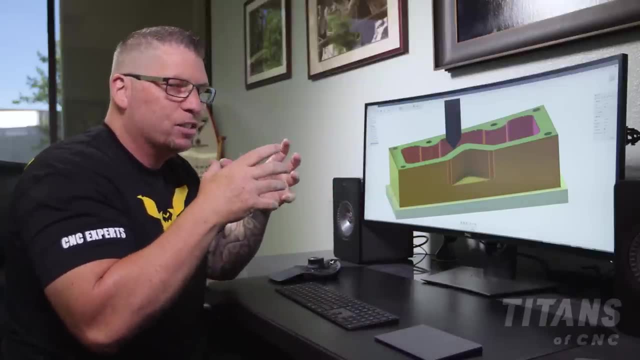 That's another thing in Inconel Right With a 6 flute tool And if you're running down here in your next tool wall, We're actually going to call it And say it's a much bigger tool So we can actually use the top. 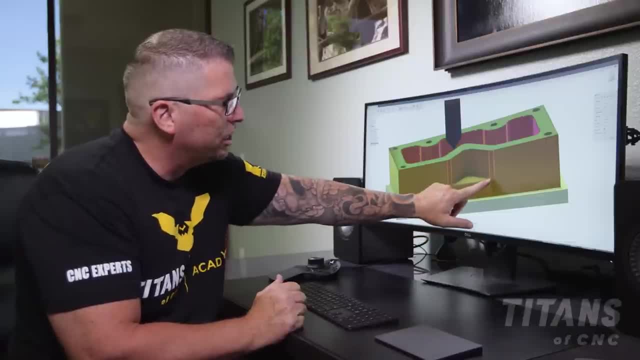 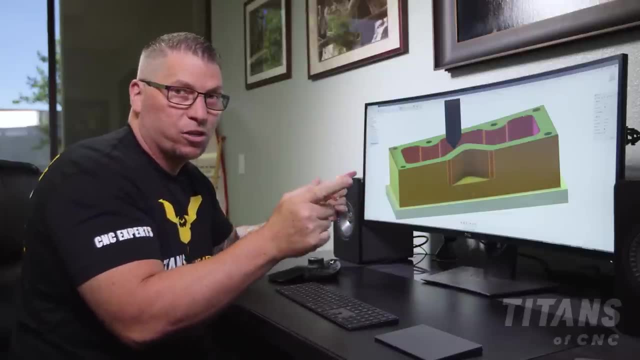 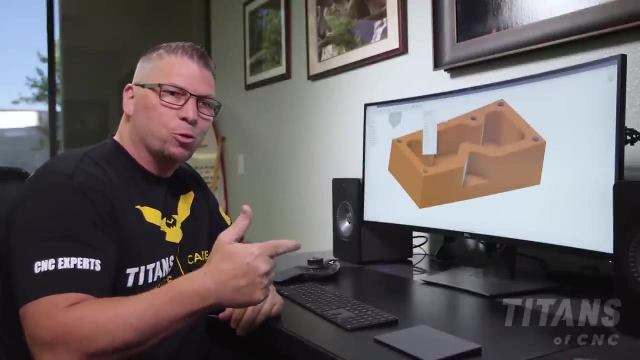 So we can get it close to the wall, Leaving the biggest chamfer, Biggest chamfer possible, Because we want to chamfer everything inside the machine, Especially when it comes to Inconel. Alright, So speeds and feeds For our Duolock 6 flute, 5 eighths chamfer mill. 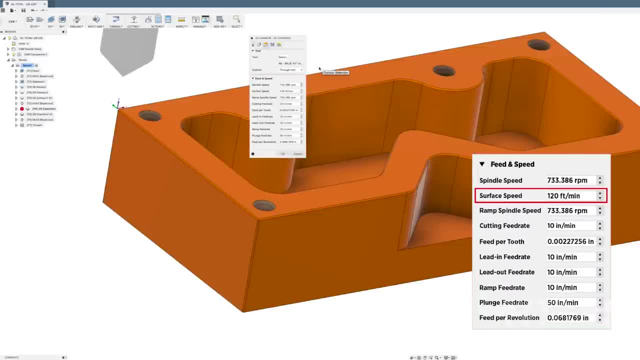 We're going to go 120 surface foot And then our chip load Our feed per tooth We're putting at .0022.. Which puts our revolutions At 733.. And at a feed rate of 10 inches per minute. Alright, 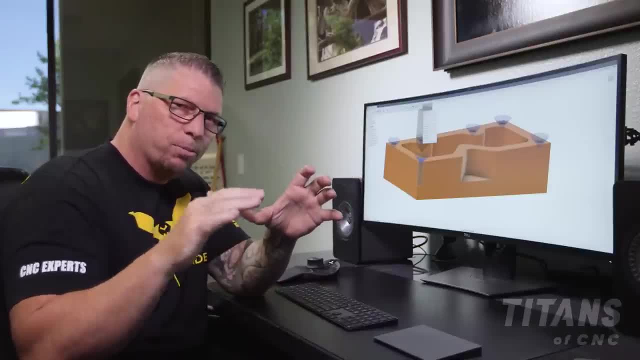 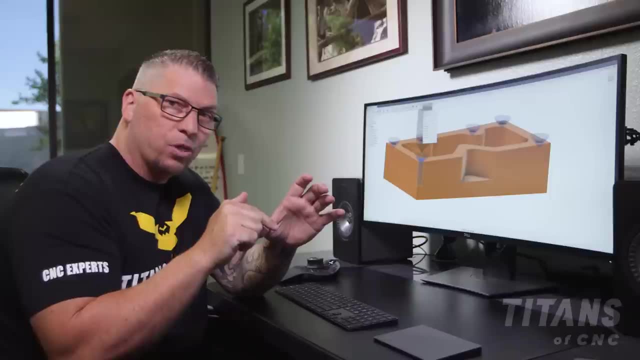 So now the chamfer mill Has actually walked around the part, Inside the part, Deburred everything, And it's going to chamfer The drilled holes now. Alright, So it's going to come straight down. So one thing I'm going to do: 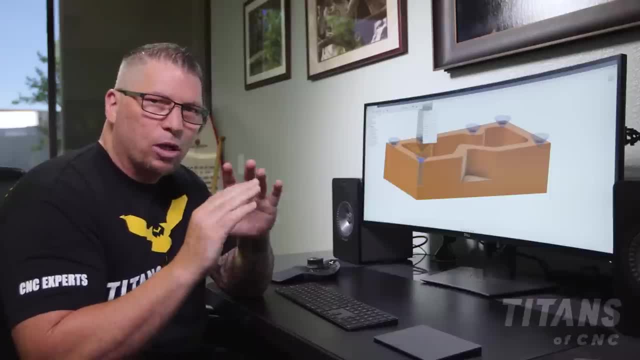 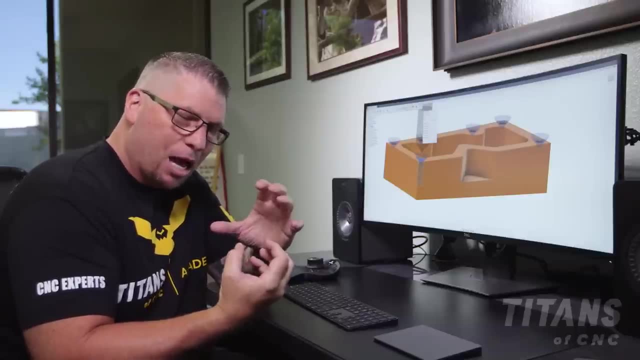 Is I'm going to actually back off my RPMs Because I don't want any chatter When this thing hits, When it hits the full diameter And it starts taking that big cut. I want to keep my RPMs low, So I create pressure. 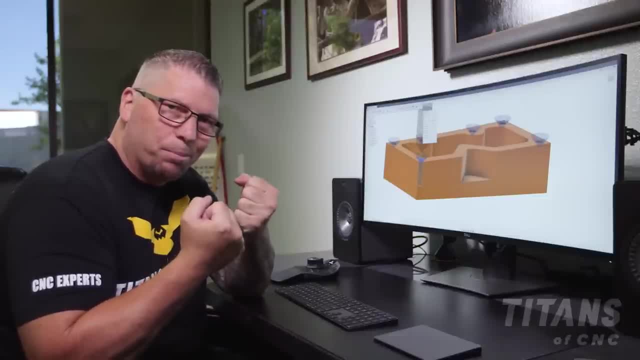 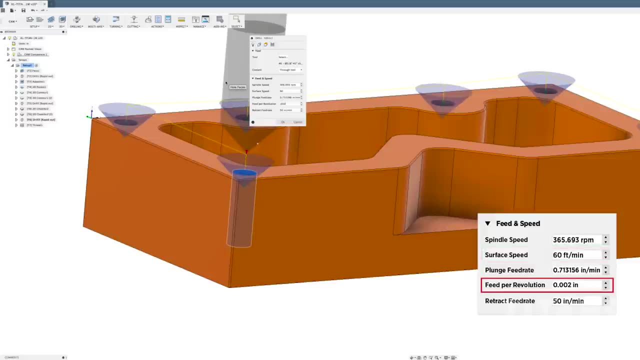 So the tool engages the material And it doesn't bounce Alright. So we're going to start off With a surface footage of 60.. And a feed per revolution of .002.. It's going to drop down, It's going to be slow. 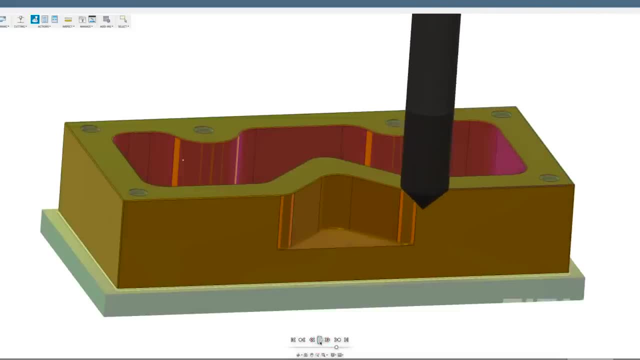 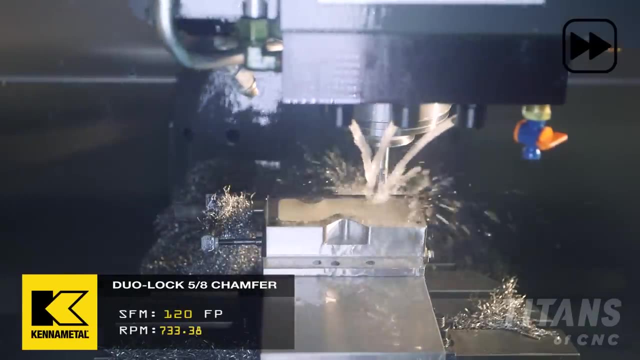 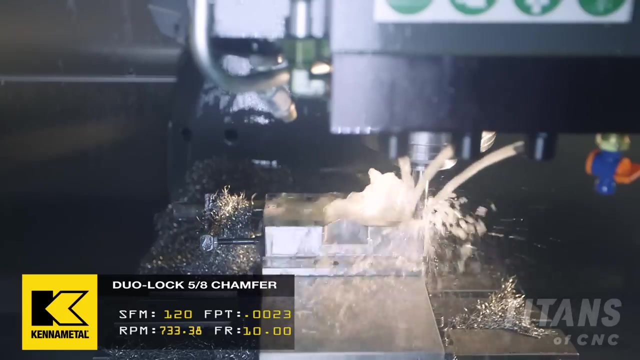 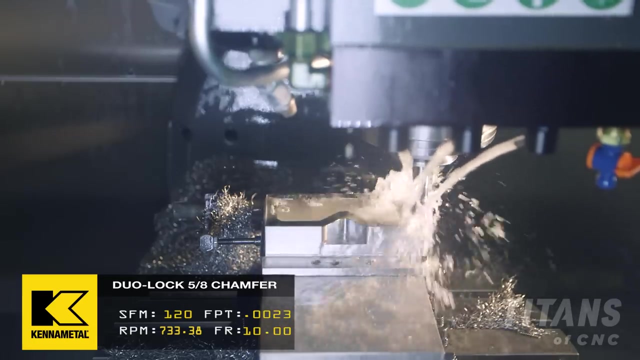 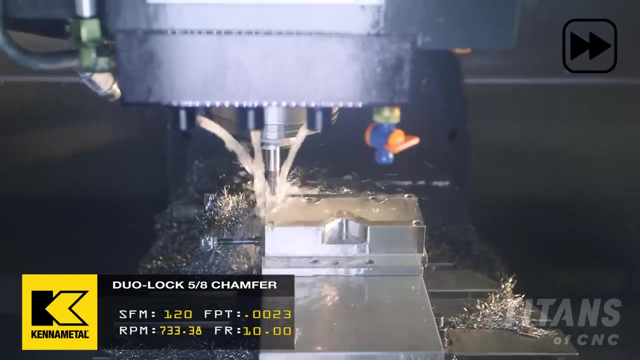 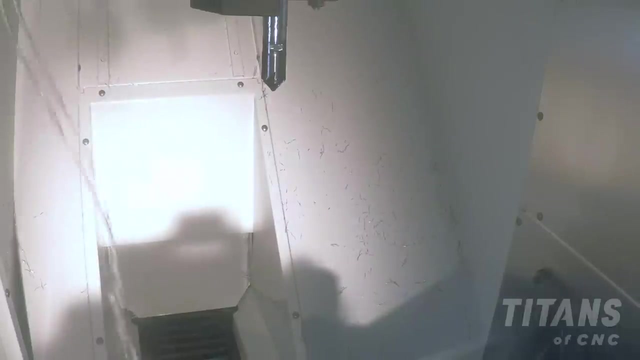 But it's okay Because it's Inconel And it's going to make a perfect finish. Alright, So we're on our last And now. the last thing we're going to do Is we're going to thread it, But I'm not going to use a tap. 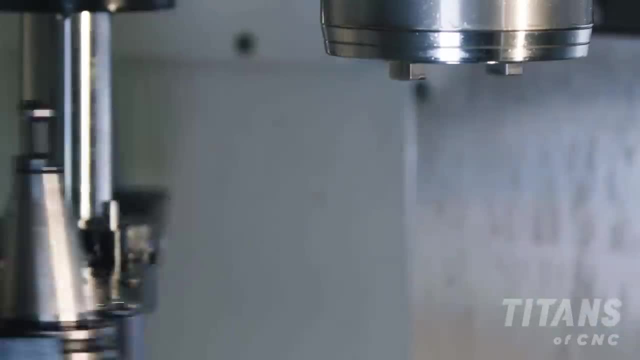 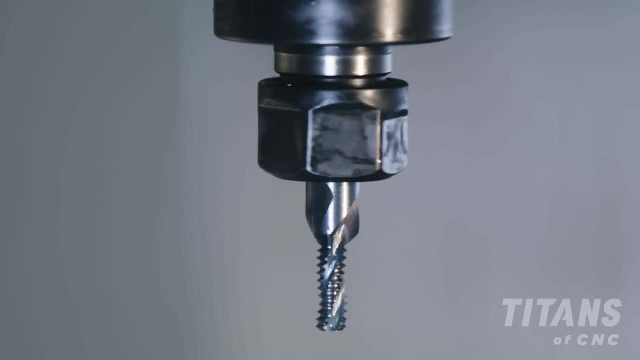 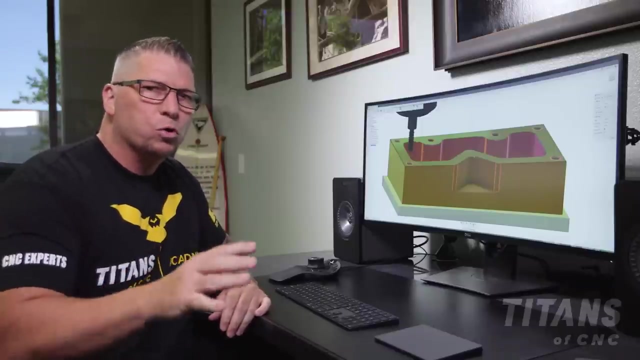 I'm going to use a thread mill, So this is a great cutter. It's designed well And it actually gets the job done quickly And perfectly Alright. So if it's aluminum Or steel like 303.. Something soft- I will roll, tap it. 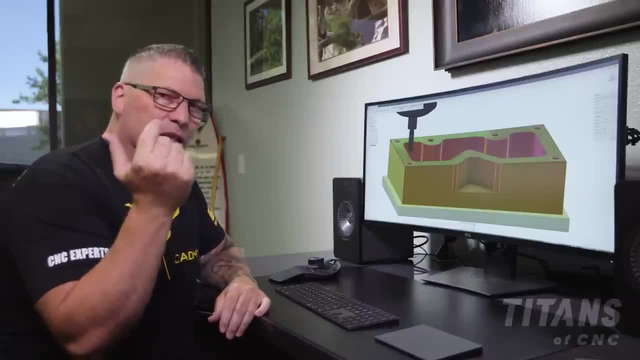 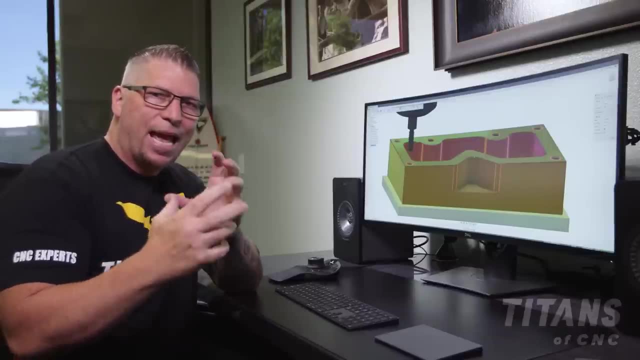 Or cut, tap it Depending. But I love thread mills Because thread mills You can comp them Right If you have a certain amount of plating, Or if it's getting etched, Or if they're calling out the size. 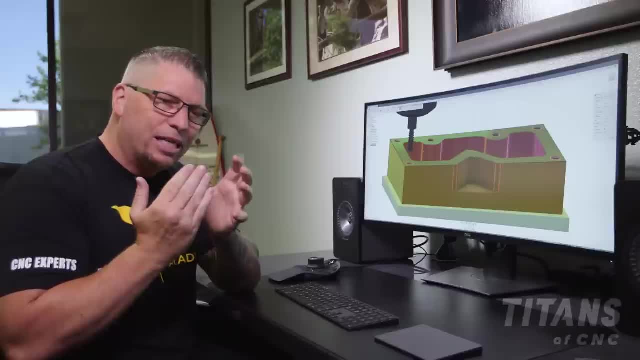 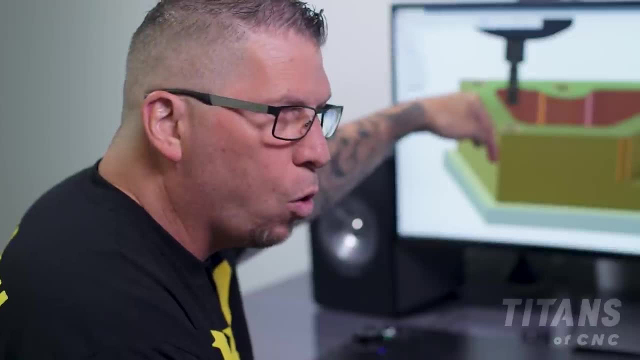 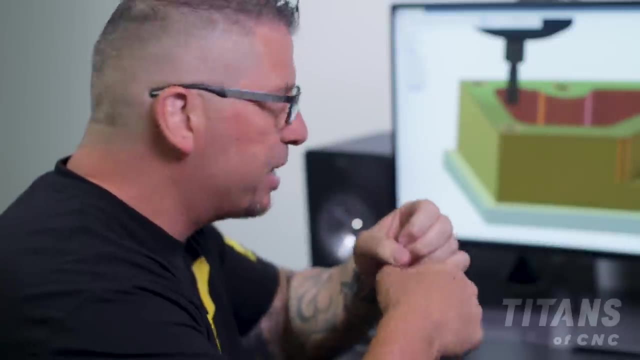 You know larger Because they're putting in an insert. You can literally adjust that thread Perfectly. And not just that: If a thread mill drops into a hole And breaks, The thread mill is smaller than the hole Right, So it usually breaks clean up at the neck. 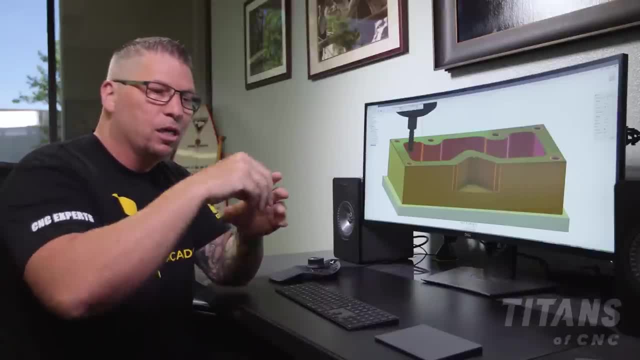 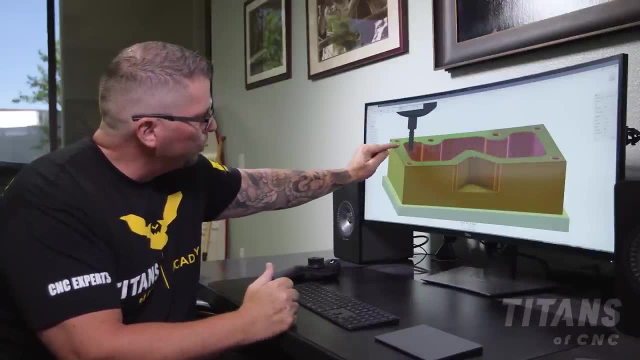 Which allows you to simply stop the machine. Take out the thread mill, Put another one in, Because it's a thread mill And the tip to the first thread is perfect. You simply can just re-probe it Or re-zero it. 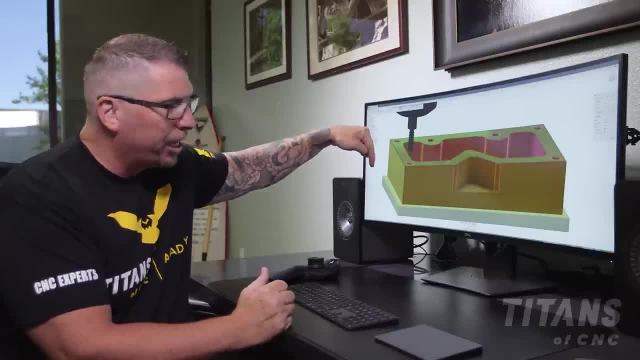 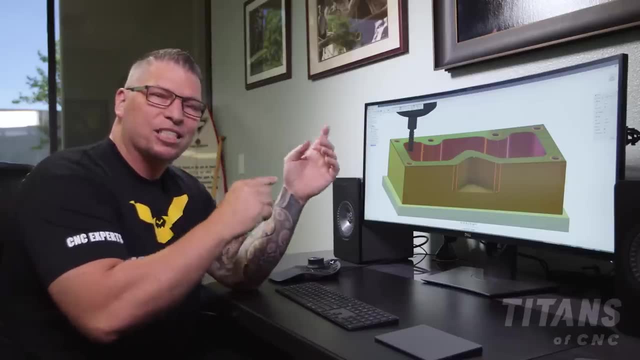 And the thread mill will drop down. Actually, pick up the exact thread. Now there's a lot of flutes on this thread mill And that's because the thread mill is specifically designed For a 5, 16ths, 18 thread. Alright, 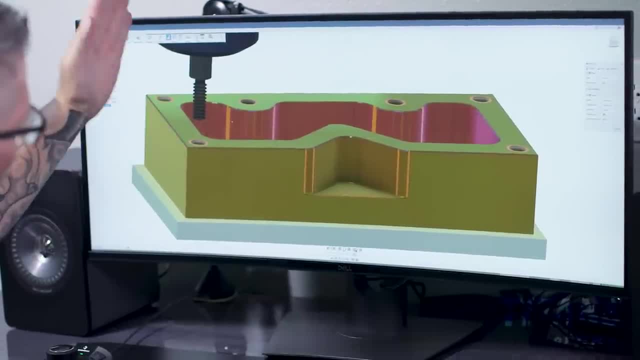 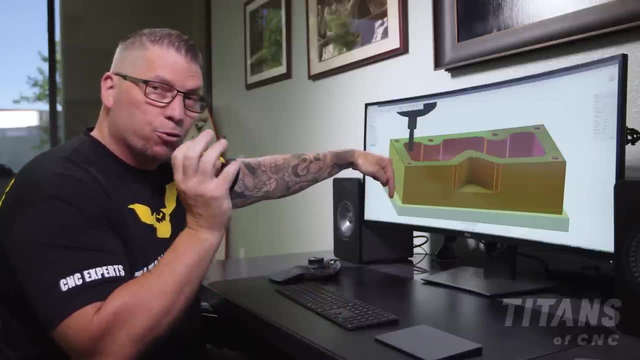 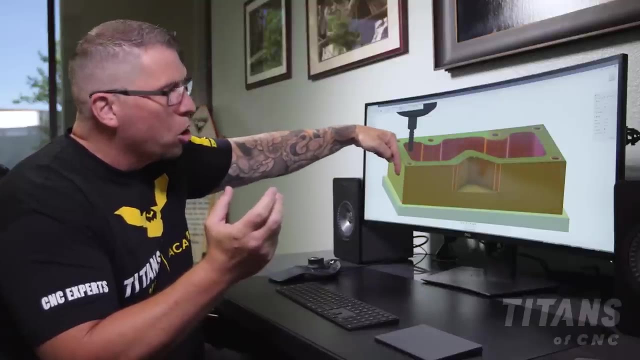 Because it has so many teeth. This thread mill, when it's spinning, Will simply drop down, Move into the major diameter Of the thread, In this case a diameter of 5, 16ths, And then it will helical up One time. 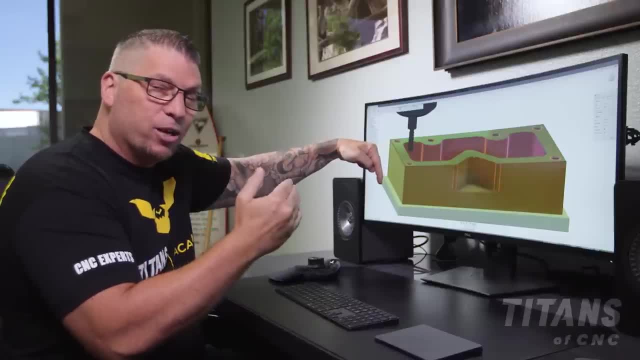 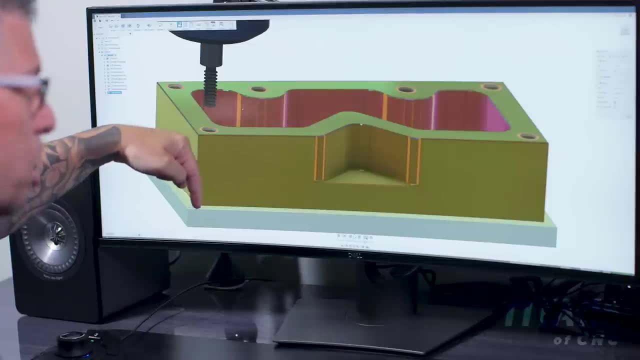 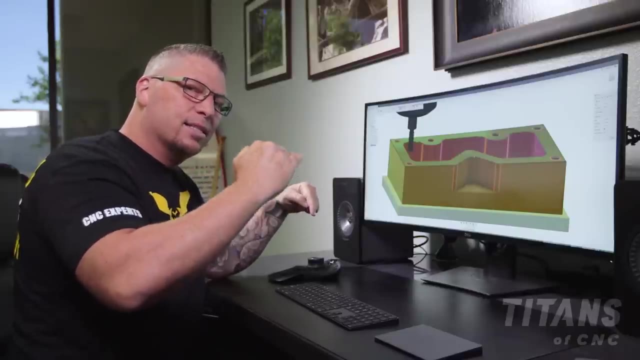 For one thread. So it's 18 threads per inch. So if you divide that That would be 55 thousandths. So it simply goes in And as it walks around That major diameter At 360 degrees, It raises at the same time. 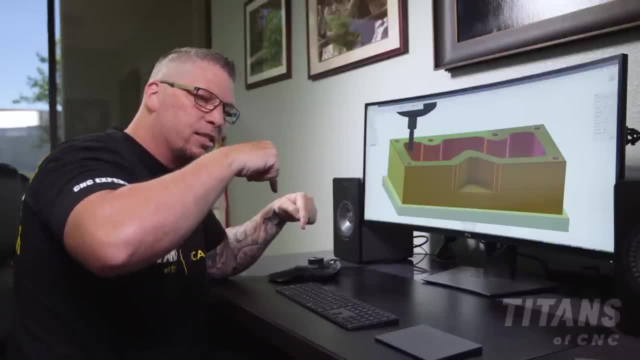 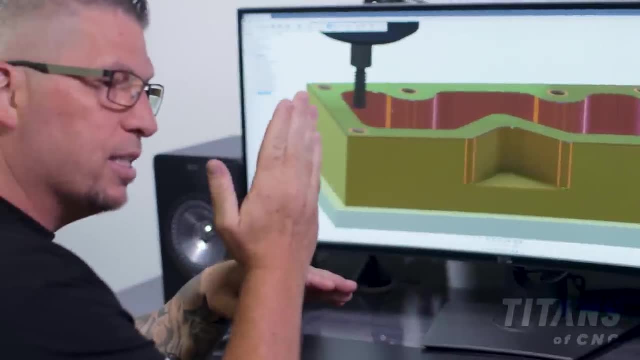 As it's going around. So by the time you hit 360 degrees, Your Z has lifted By 55 thousandths And then the tool will disengage. Then, through the entire diameter of the hole, All of your threads, All the way up. 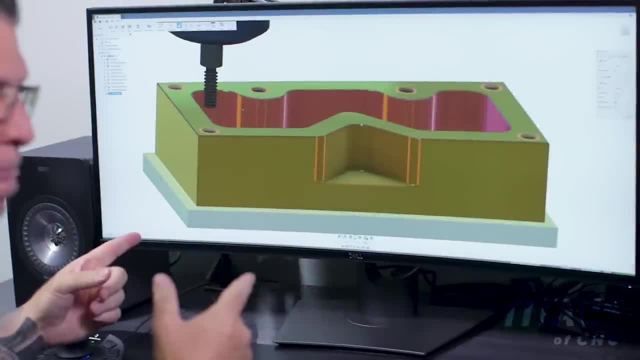 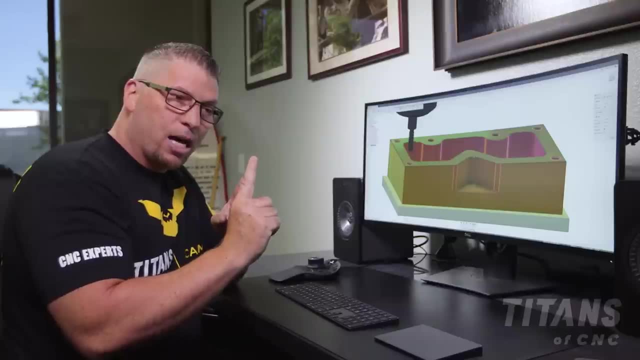 Will be perfectly cut. So, since this is Inconel, I'm going to walk in. I'm going to leave 5 thousandths And do one roughing pass. I'm going to come out. I'm going to drop back down. 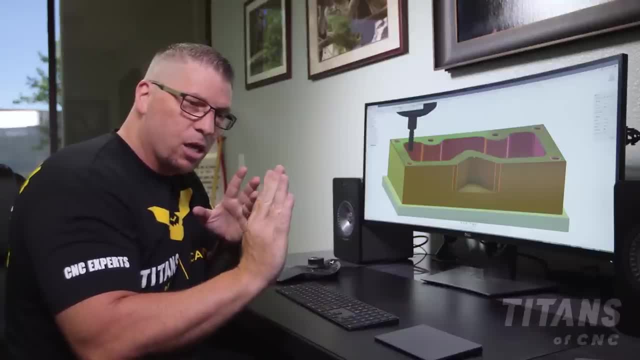 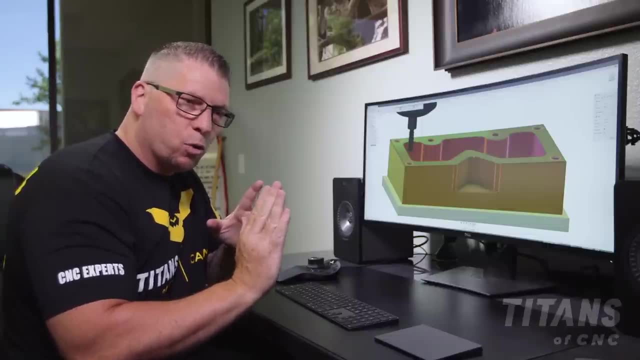 I'm going to walk in that extra 5 thousandths To do my finish. I'm going to do it one more time And then I'm going to come out, Go down. I'm going to do it one more time, Just as a spring pass. 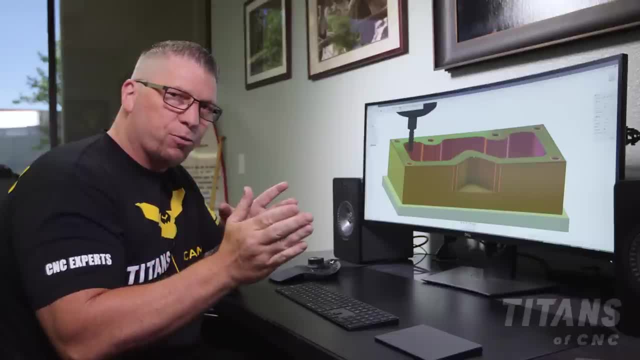 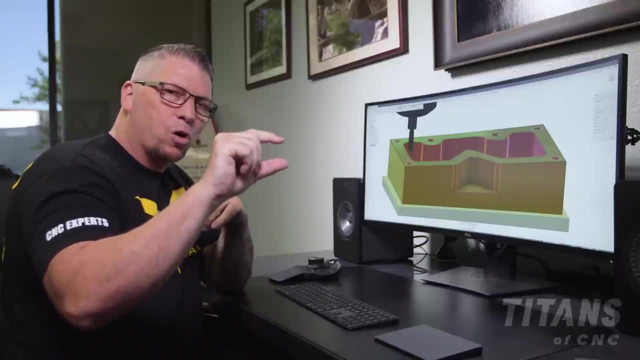 Not to take any material, But just to make a perfect thread And catch any material that's left Because the tool might have deflected, Because it's hanging out so long In Inconel. Alright, So let's do this. 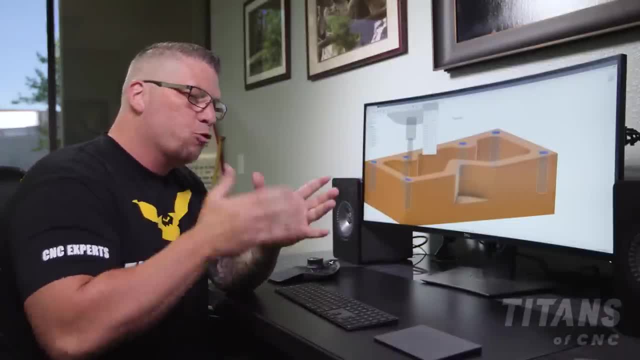 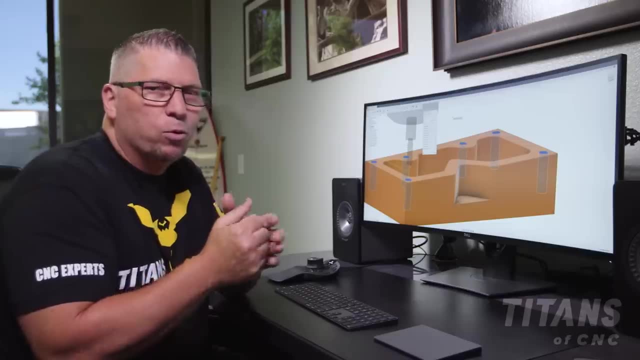 So one of the cool things about the thread mill is You would think that you would drop down And just like inch around it Like .5 bead rate Or something very delicate and very small, But we're going to actually get after it a little bit. 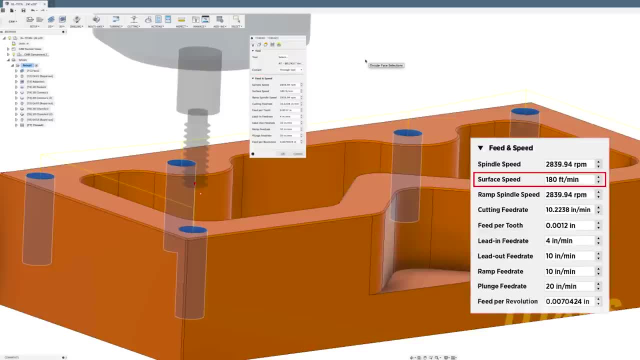 Okay, So our surface footage is at 180.. Alright, That's a good surface foot right there. And then our feed per tooth is at .0012.. This is a three flute tool, And that's going to put us at a cutting feed rate. 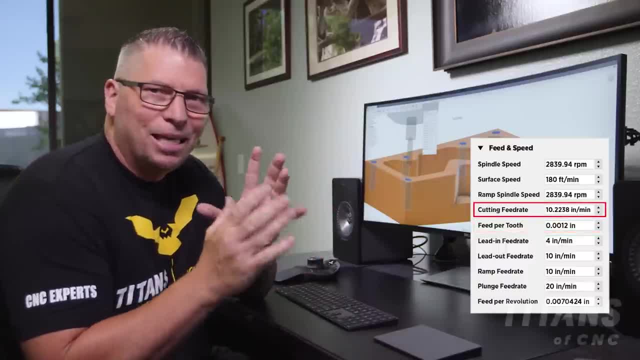 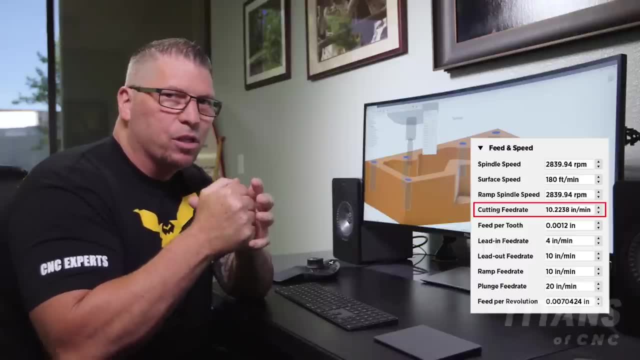 Of 10 inches a minute. 10 inches a minute doesn't seem like a lot, But when you're dropping down And you're only moving out like 50 thousandths, You get there quick, Right. And then when you move around in that small little space, 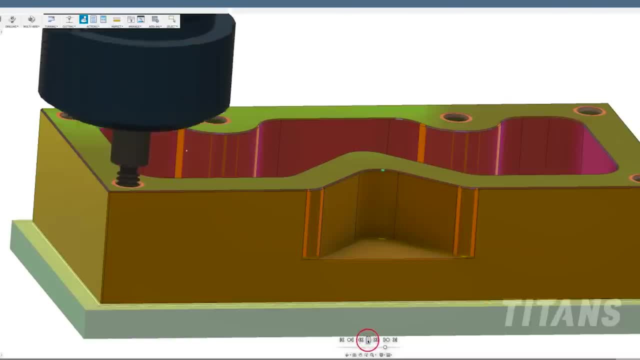 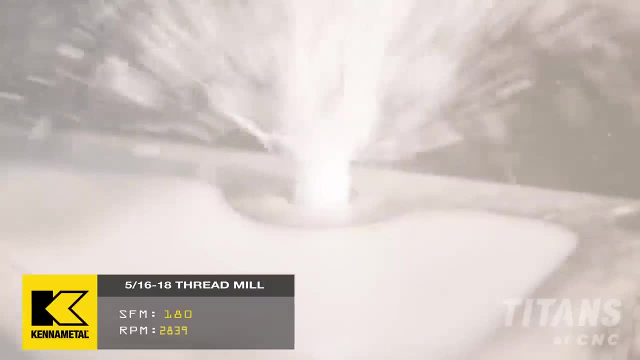 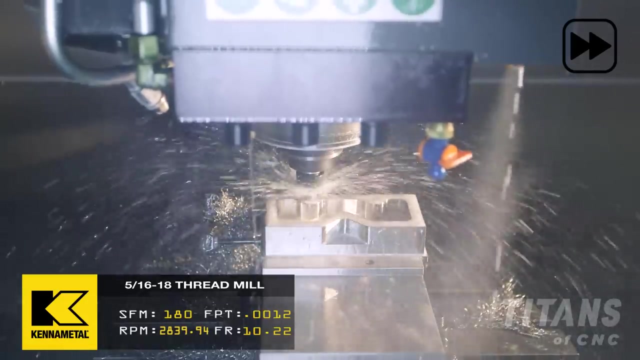 It moves quick So it's going to go in, Boom Out, In, Boom Out. The tool actually has a hole going through the tool So coolant actually comes out the bottom. It flushes those chips But because the diameter is .257.. 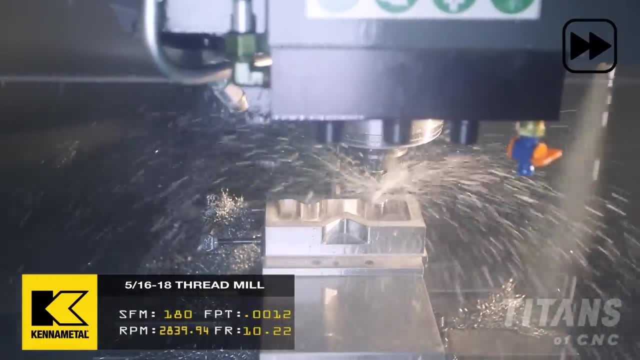 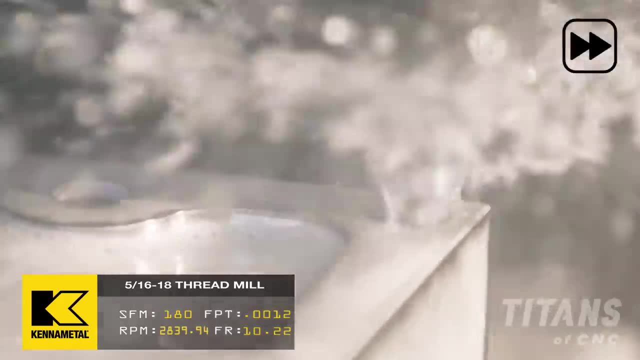 And the tool is .242.. There's not a lot of space, Okay, And I don't want to run those chips over. So what I'm doing, with an understanding That it's flushing the bottom of the hole, Is I'm lifting up. 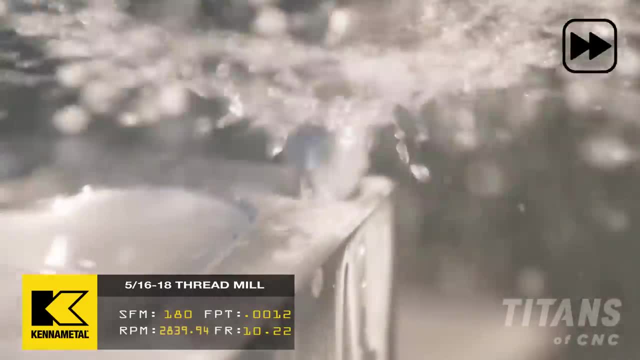 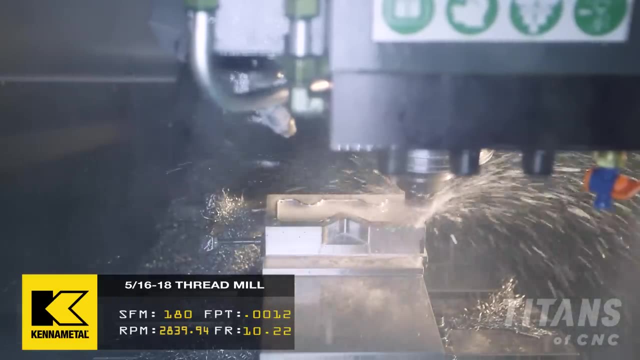 As I'm lifting up, It's flushing the bottom, It's pulling all the chips out. So by the time I come up, All the chips are out, And then I just drop back in, Walk around again, Come out, Drop back in. 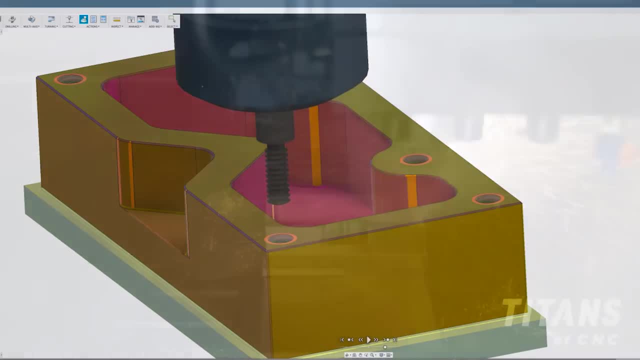 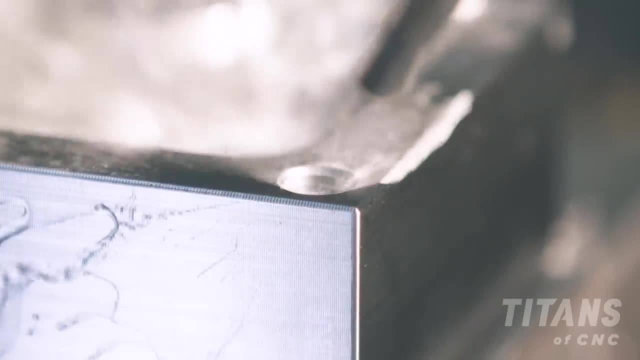 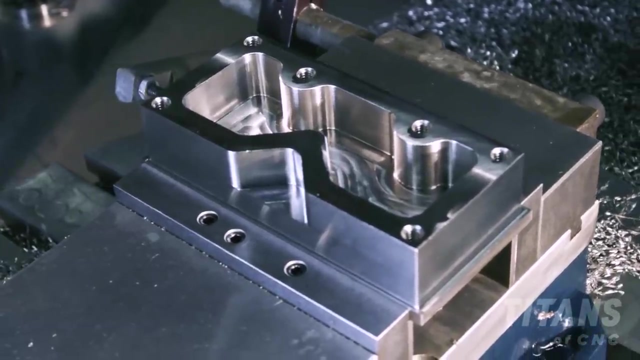 Do my spring pass Come around For a perfect finished thread? There we go. Check it out, The Titan 1M Extra Large Inco version Right there. So check it out. You can actually look at all the surface finishes. 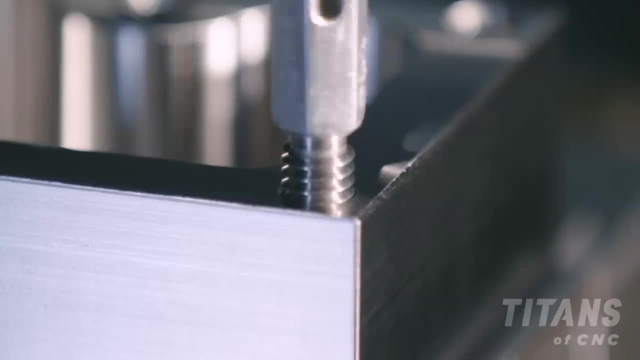 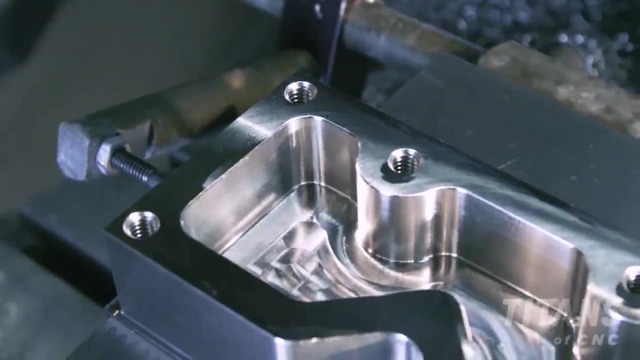 Everything looks absolutely perfect. We put the thread gauges in The go, the no go. Everything is absolutely perfect. The finish is nice and smooth All the way around. Part looks absolutely beautiful. We haven't done any external finishing or deburring. 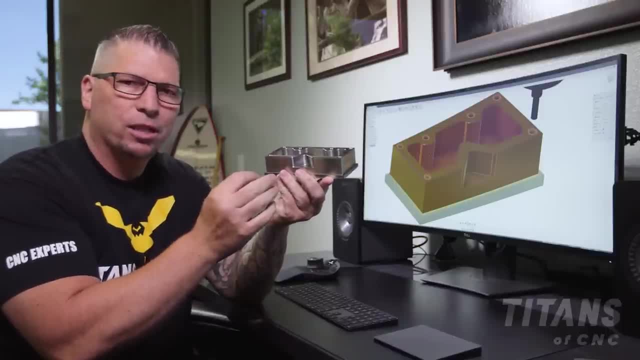 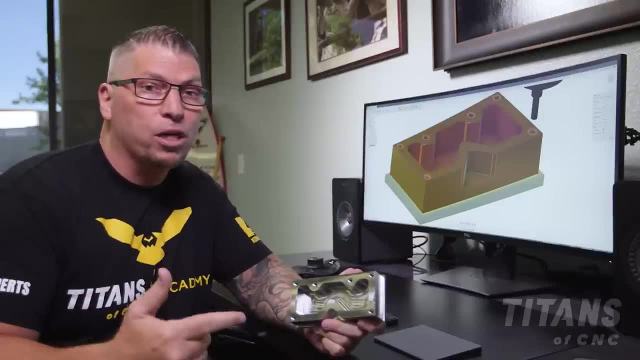 That is exactly how it came out of the machine. I hope you guys learned something And if you love this video, Please hit that subscribe button below Because we have a whole bunch more Just like it coming. CNC machining Ink and L.